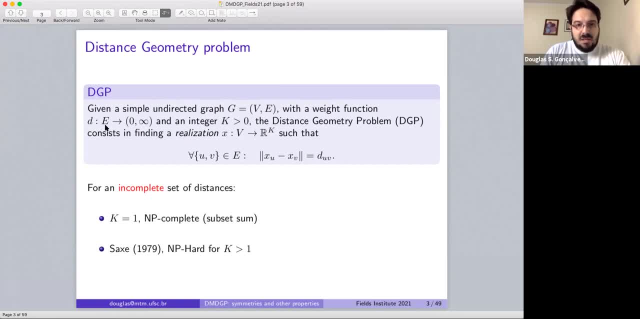 associates positive weights to the edges of this graph. and we have an edge in this graph if the distance between two vertices is known, and an integer k which is positive, which represents the target dimension. we'd like to find what we call a realization, so a map from the set of vertices to Euclidean space of dimension k. set that to the – that we call a realization, so a map from the set of vertices to Euclidean space of dimension k. set that to a dimension k and then set that to the distribution of the partition of the dimension. When the dimension k is positive, we will cannot find a distribution of the variable. 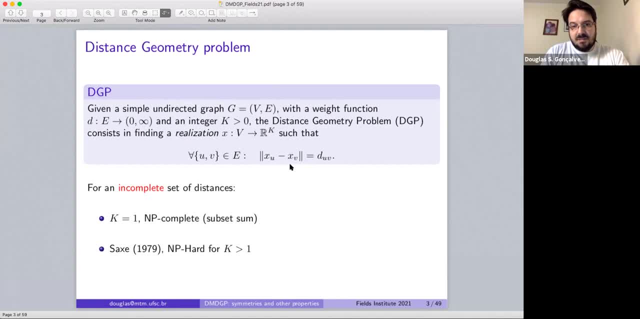 they realize that the distances, the Euclidean distances, coincide, match with the given distances. So this problem is known to be NP-hard. It was proved by Sachs. For any dimension K, in particular for dimension K equal to 1, it is NP-complete. And Leo Liberto gave 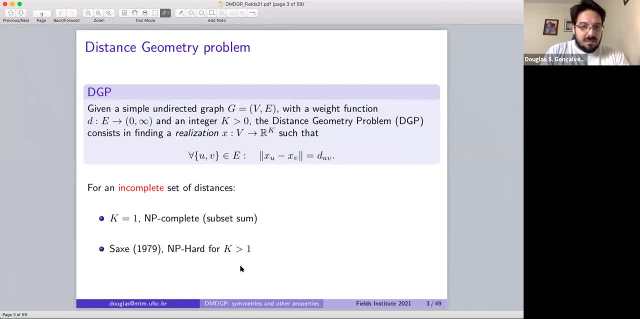 an explanation in his talk on Tuesday. You can show that by polynomial reduction from partition or subset sum. But there are special classes of this distance geometry problem for which you can obtain polynomial time algorithms. For instance, if you have all the distance which means that your graph is complete, then you can obtain the realization by performing: 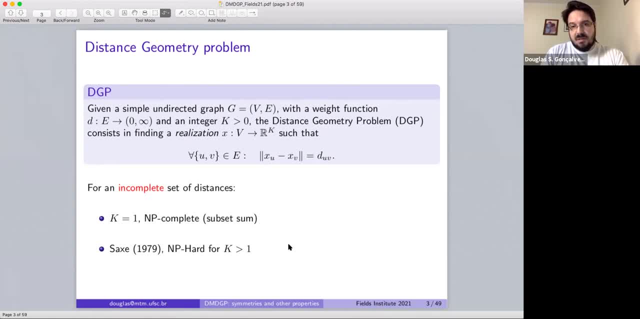 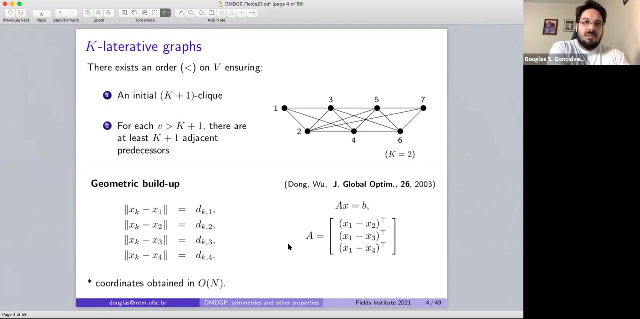 the spectral decomposition of the grand matrices, a grand matrix associated to the distance matrix, when you have all the distances. But even if you don't have a complete graph, you still have some classes of this problem for which you can solve the problem: polynomial time. One of these classes is what we call decision problems, where the 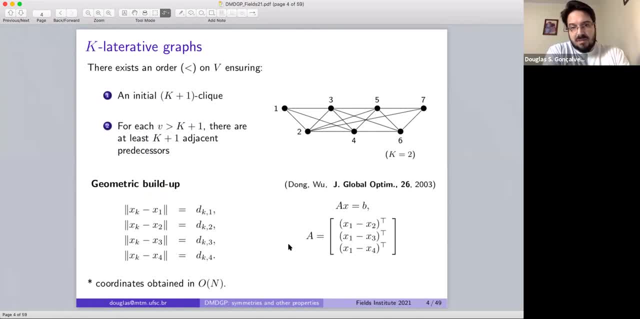 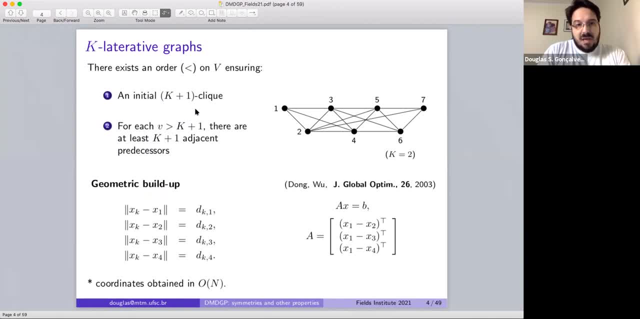 find an order for the vertices. You can find an order for the vertices. You can find an order for the vertices of this graph such that the first K plus one vertices form a clique and for all other vertices, ranked after vertex K plus one, there are at least K plus one adjacent predecessors. 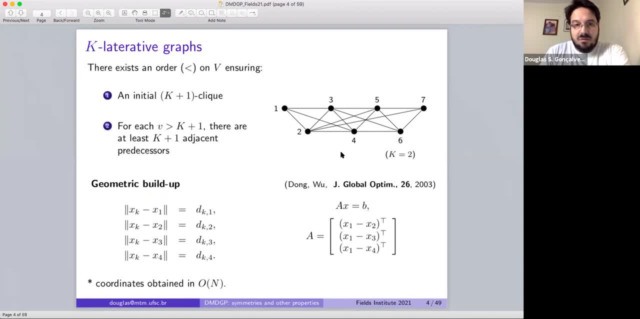 So here on the right I give an example for the dimension K equal to 2.. So this graph: you can consider here the vertices 1,, 2, 3 forming a clique, and then you see that for all vertices 4,, 5,, 6,, 7.. 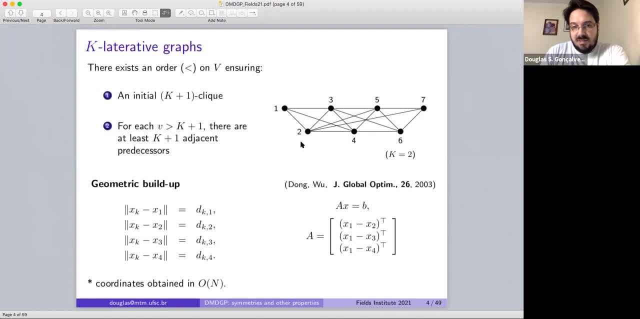 there are at least three adjacent predecessors. And why is this property good? Well, this property is good because it allows us to perform K-lateration, which means the following: If you are working, for instance, in dimension K, equal to three, okay. 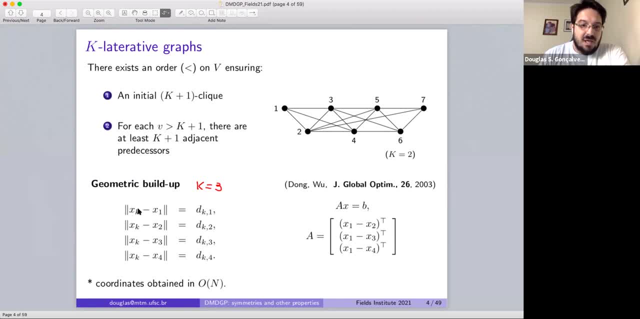 And we would like to find a position for the vertex K, And we know it is adjacent to vertices one, two, three and four. okay, Then the position for the vertex XK can be obtained by solving the system of quadratic equations. Actually, we can put this square here and there, okay. 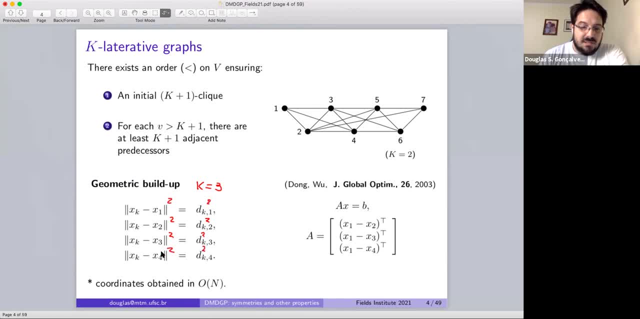 And it turns out that this system can be reduced to a linear system for which the matrix A is non-singular as long as the points X1,, X2,, X3, and X4, which are positions for already localized vertices, can be obtained. 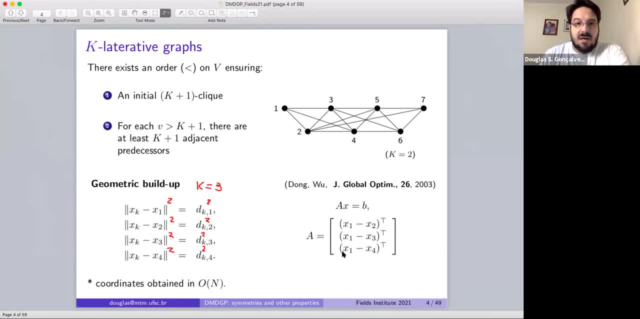 One, two, three and four, as long as they are affining independent. In this case, in dimension three, the four points do not lie on the same plane. okay, In this case you can compute all the vertex positions in linear time. 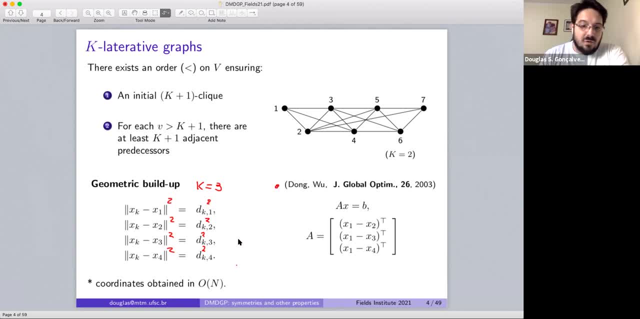 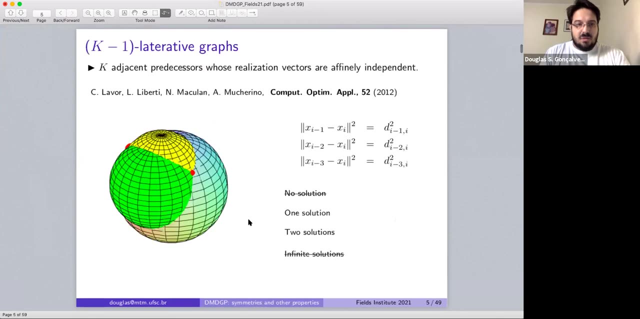 And this is a work from Vu, from Dong and Vu. okay, Of course, here we are considering exact distance. all right, Another class we are going to do is a class of graphs, for which we can do some things in this direction, is what we call. 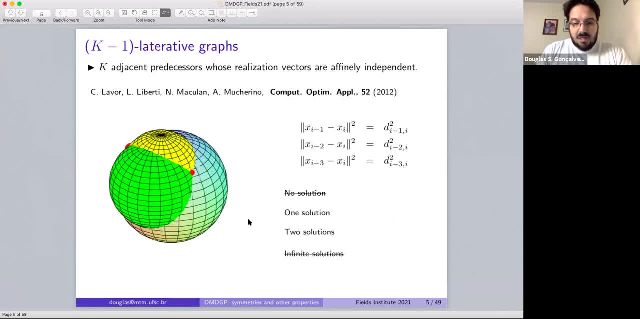 the K minus one alternative graphs. In this case we weaken the assumptions a little bit. Instead of asking for K plus one adjacent predecessors, we ask only for K. But then, instead of performing the intersection of K plus one spheres in our K, which in general gives you 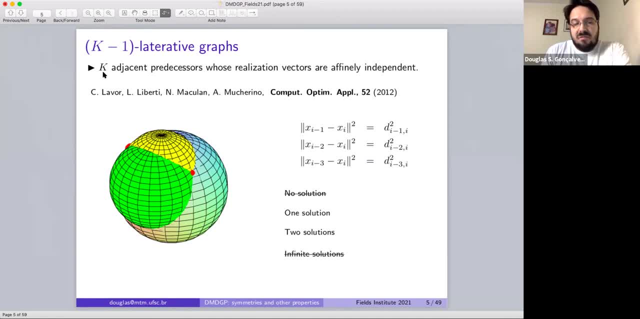 only one position. we are now performing the intersection of K hyperspheres in our K, which, under sweet ball assumptions, can give you at most two solutions. okay, So the possibilities are: the intersection of this. K spheres could be empty, one point, two points or infinite points. 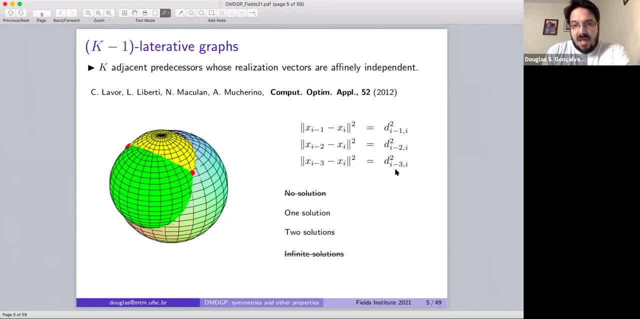 But if we suppose that the instance at hand is IS instance, which means it has a solution, then we rule out this option And if, as long as the vertices, the predecessors: okay: X, Y minus one, Y minus one, Y minus three. 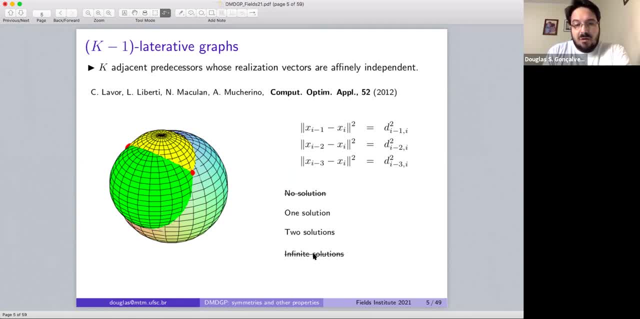 are not collinear, then we also rule out this last option And we end up with one or two solutions, okay, So I will focus in this talk about this kind of distance geometry problems, okay, For which then they're like: this is a K minus one alternative graph. 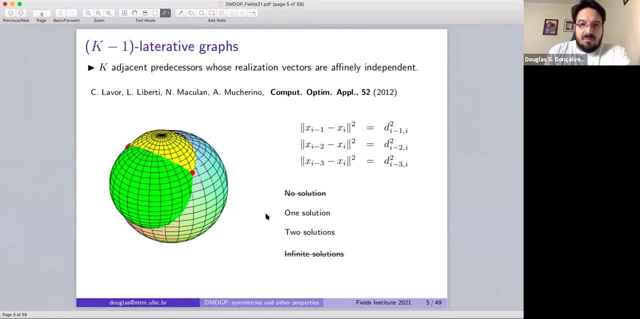 In this case, of course you are imagining okay, but if I have two points, which one should I choose? And we'll see that actually, in the sequential approach that we consider, we just call it branch and prune, We actually consider both, okay. 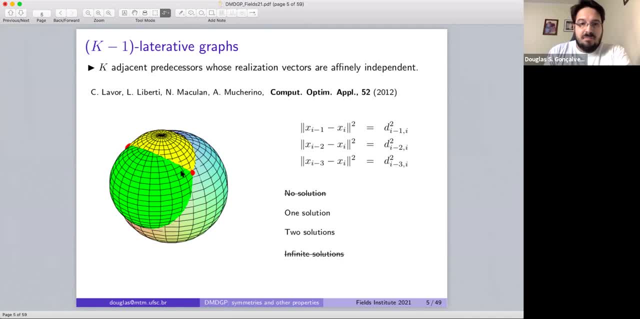 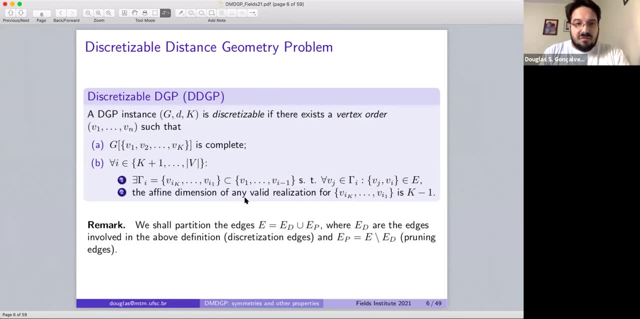 And this leads to a binary tree of possible positions. So based on these ideas of K minus one lateration, I define now what we call discretizable distance geometry problem. So we say that the distance geometry problem is discretizable if there exists a vertex order. 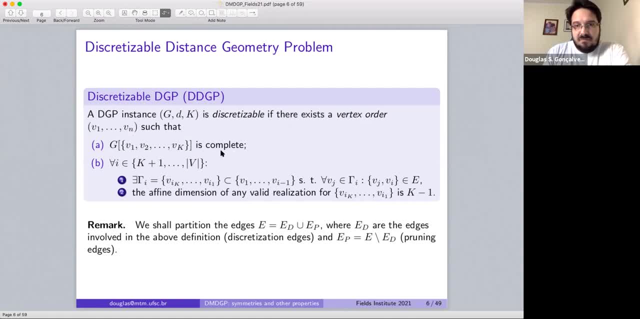 such that the first vertices, in this order form, a clique, as I said before, And we have the following For each vertex from index K plus one to index N or cardinality of V, the vertex VI must have at least K adjacent predecessors. 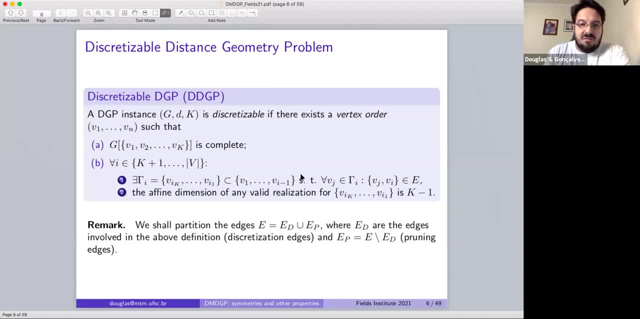 So this ugly expression here just means that VI must have at least K adjacent predecessors, And moreover, the position for these K adjacent predecessors should have a finite domain, a binary dimension, K minus one. So if we're working in the plane, for instance, 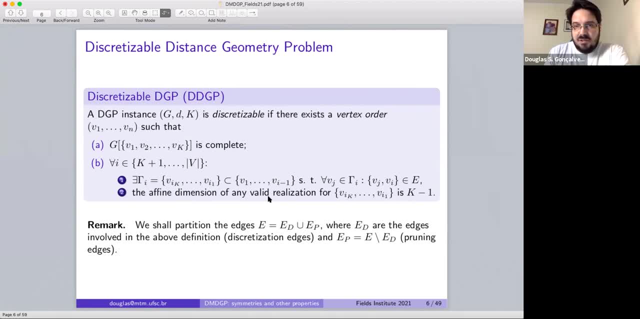 it means that the two points cannot be at the same position if we're in our tree, So the three points cannot be collinear, and so on. okay, It's important to notice that in this definition we involve only a subset of the edges in the graph. 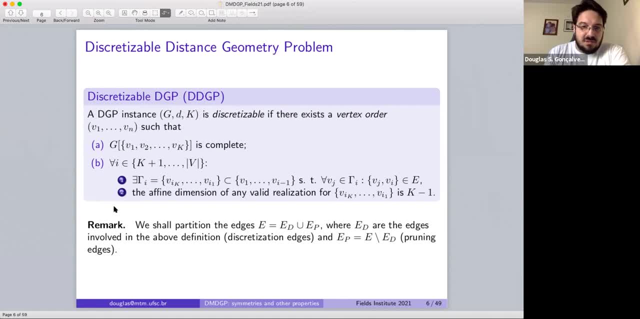 or you consider a subset of your distance constraints that we're gonna call discretization. edges Are the edges involved in this assumption And we will represent them by EG. and we have all the others that we may or may not have. we call the pruning X. 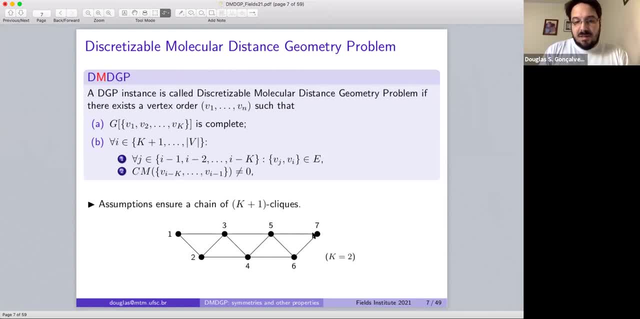 And in fact I will consider a subclass of the DDGP which we call the DNDGP. So we have a set of two vertices where we change the second assumption and we ask the adjacent predecessors to be contiguous. We asked to immediate adjacent predecessors. 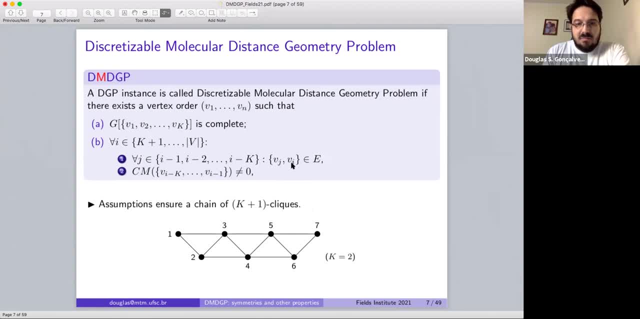 So for each vertex VI with I greater than K, it must be connected, it must be adjacent to the vertex I minus one, I minus two, I minus K. And if you have this condition we can we write the second condition where we ask the positions. 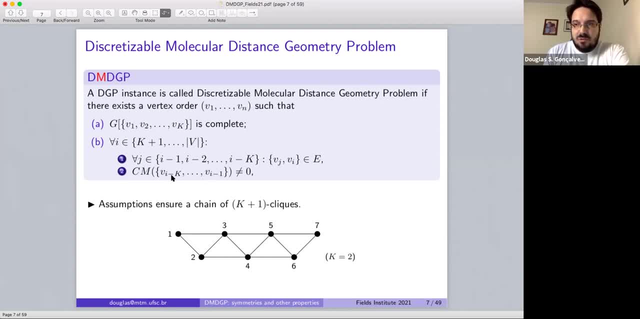 for these vertices to lie in an affine space of dimension K minus one. We can rewrite this condition using the Cayley-Manger determinant, asking the Cayley-Manger determinant to be non-zero. And well, so this N here stands for the molecular. 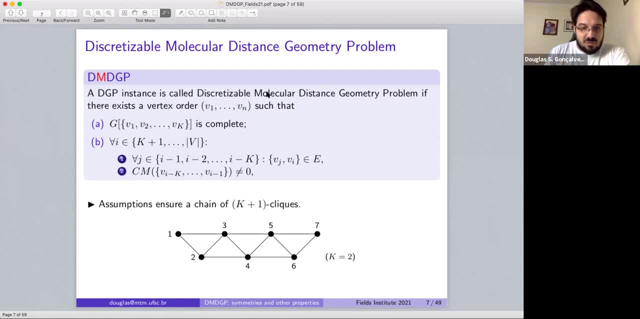 because this class of distance geometry problems appears often in the context of protein structure determination, And so we include this M to stress the fact that the adjacent predecessors must be contiguous. Okay, In this definition, it implies what? in terms of the topology of the graph, 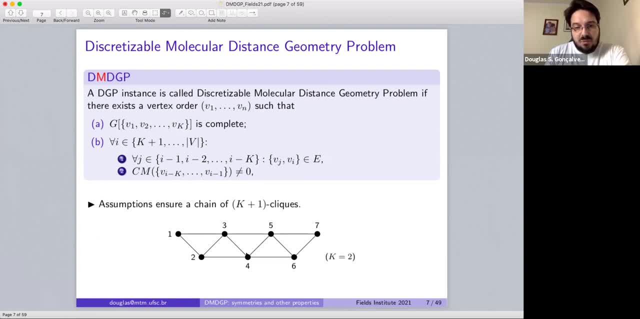 it implies that the graph is a chain of K plus one clicks, like this one I showed here. Okay, Of course one may ask: okay, but how do we know that? How hard is to determine if such vertex order exists? And this talk will be discussed in the next talk by Merv. 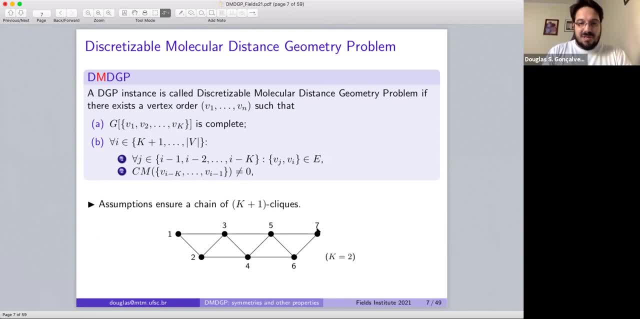 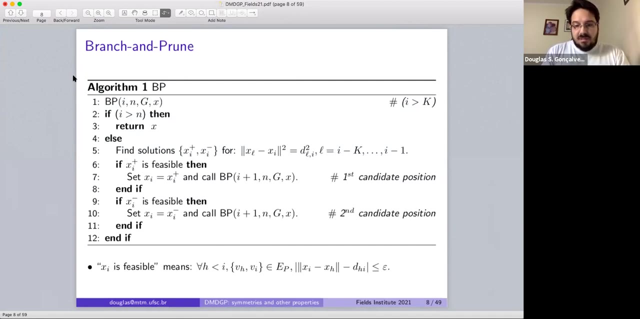 Okay, So I will leave with her the discussion about how to compute the vertex orders. From now on we will discuss about this class of problems, the DMDGPs. So for the DMDGPs, we can exploit the search space. 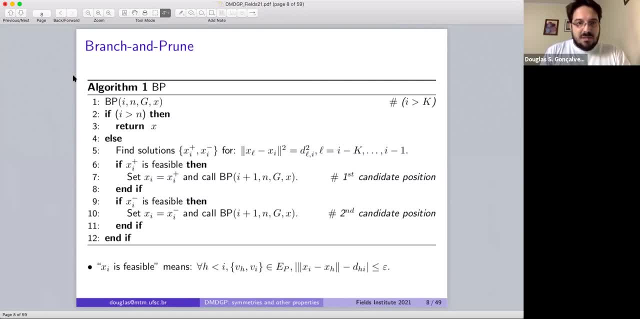 which is represented by by a binary tree, using an algorithm called branch and prune. Here I show up pseudo code for this algorithm, which is showed here in its recursive form. Okay, So the algorithm calls itself recursively, given the initial positions for the first K vertices. 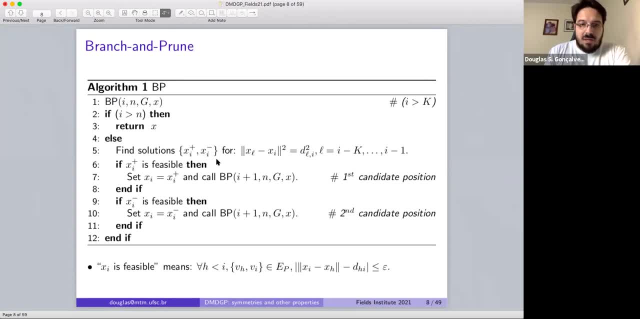 for all other vertices. what we do is the following: We, the assumptions- ensure that we have at least K adjacent predecessors, So we perform intersection of K spheres and RK by solving this quadratic system. Okay, And this generates two possible candidate positions. 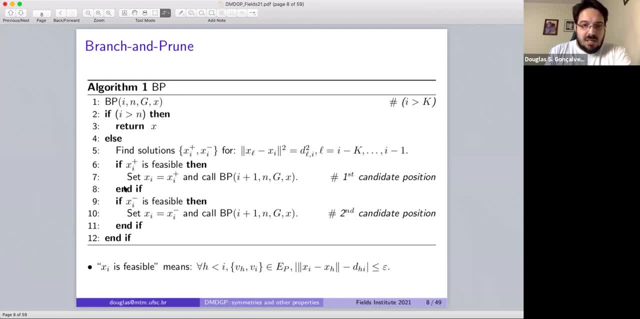 Okay, I call it here XI plus, XI minus, And then we check the feasibility of each position. If it's feasible, then we continue. We call the branch and prune in the next vertex Okay, Otherwise we go to the. 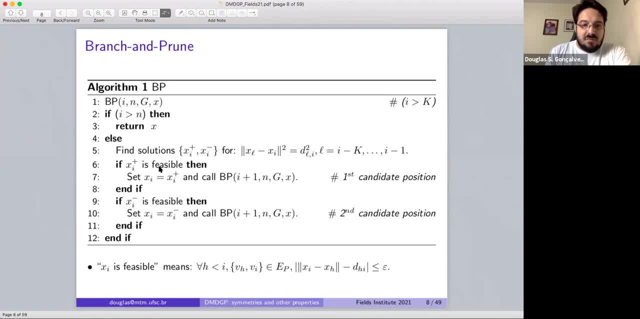 to the other candidate and try again. And here by feasible we mean the following: We mean that all adjacent, all edges Okay, Related to adjacent vertices to neighbors of VI that were not used in this quadratic system, They are verified. 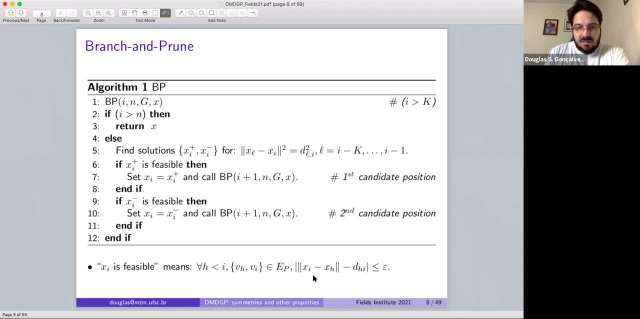 And we say that the XI is feasible if the constraint related to the distance GHI is satisfied with. Roozbeh Gharakhloo: Tolerant within a tolerance, excellent, okay, actually this feasibility test, you could include other Roozbeh Gharakhloo Criteria, Okay. and for instance, yesterday Jen she mentioned that some properties like the, the vendor vows constraints and so on, and so if you are working with 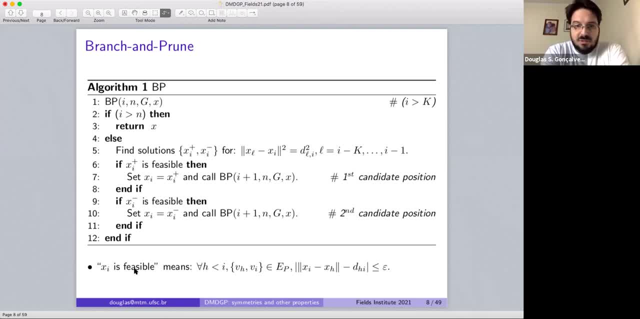 Roozbeh Gharakhloo Molecules. if you are working with the protein structure termination, you could include some other pruning devices here, for instance using information about the vendor. of all forces are also Roozbeh Gharakhloo, Q reality and so on. if you are working, for instance, with sensor networks, then you could exploit to the radio range to include their order of stability tests. okay. 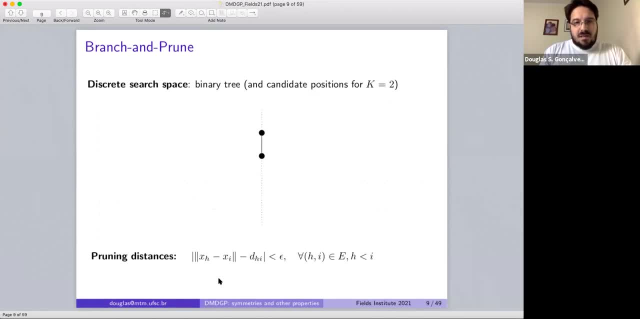 Roozbeh Gharakhloo. And here is an example of how these binary networks are working: Roozbeh Gharakhloo, Where the binary tree is built. Okay, actually the binary tree is an abstraction. okay, just to represent the possible choices that we have. 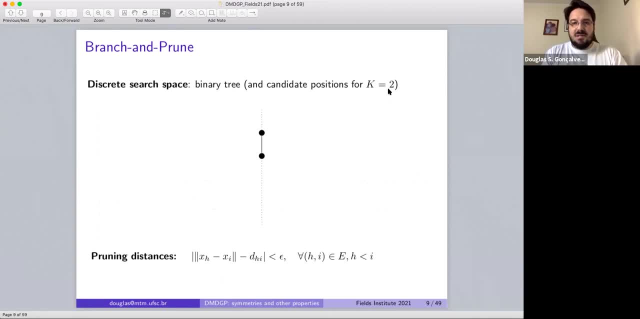 Roozbeh Gharakhloo For each vertex position, but in particular, when the dimension is K equal to two, I can draw in the same figure Roozbeh Gharakhloo, The binary tree and also the candidate vertex positions. so that's what we're going to do. so suppose, here you you have. 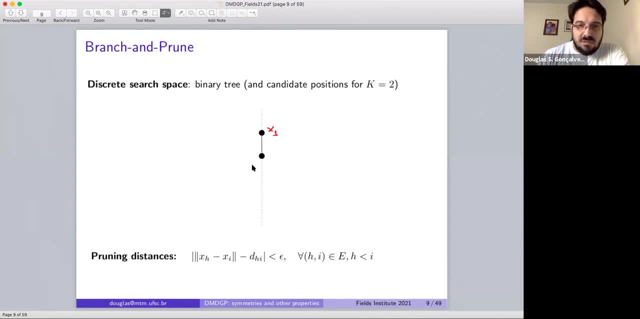 Roozbeh Gharakhloo, Your first vertex X, one that you could the place at the origin of the plane, for instance Roozbeh Gharakhloo, And then it's the vertex X two, or, yes, the distance between one and two is given by this line segment. then X two would be here and Okay, this is our initial K click. 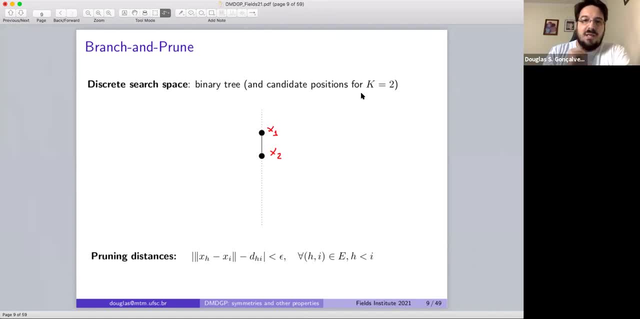 Roozbeh Gharakhloo. Okay, and then for all the other, versus the dmgp assumptions, ensure that, for instance, for vertex tree, we know the distance from Roozbeh Gharakhloo, The, the third vertex to the, to the first and the second. 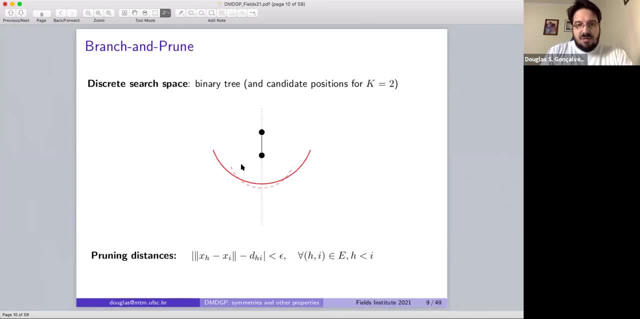 Roozbeh Gharakhloo, And then we can perform these few intersections. so here i'm representing part of these fears. okay, Center at Roozbeh Gharakhloo, One and two, and the respective ready Roozbeh Gharakhloo. And then we have these two possible positions. Okay, we consider both and then we make a choice: we go to the left or to the right. suppose we go to the left. 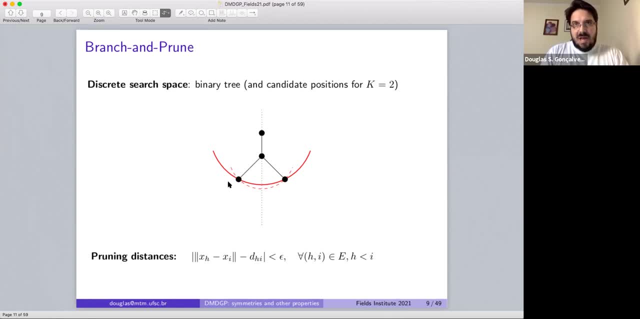 Roozbeh Gharakhloo. Then for the fourth position, the assumptions ensure that we have distance from the fourth vertex to the vertices three and two- Roozbeh Gharakhloo. And then we again perform industry intersection, and these leads to another two positions. now for vertex for. 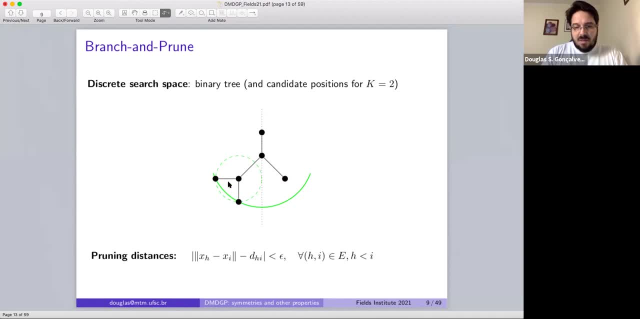 Roozbeh Gharakhloo. Okay, and we keep growing the tree in this way. however, eventually you may have more than two, in this case more than K- adjacent predecessors, and this additional information can be used to prune Roozbeh Gharakhloo In feasible candidate positions. so here are two positions for the. 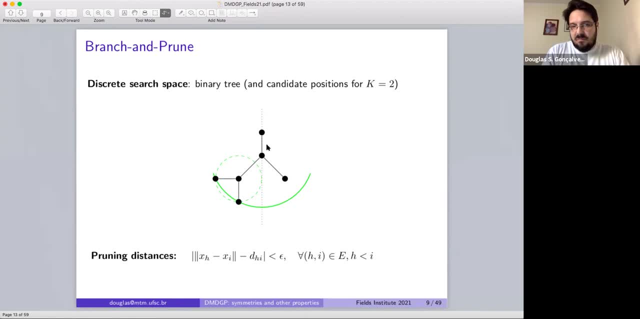 Roozbeh Gharakhloo vertex for. but for instance, if you have a distance from vertex one to vertex for Roozbeh Gharakhloo, That passes Okay, that is matched only by this vertex, then we prune this other candidate position and consider this one okay. here's important to mention that I only showed in this, in this example, this example. 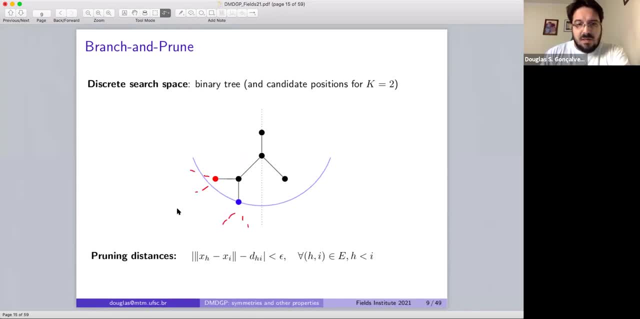 Roozbeh Gharakhloo For vertices, but district could keep growing here. of course, when you Roozbeh Gharakhloo As a certain point, you do not consider the subtree which is hooted on this vertical position. okay, and 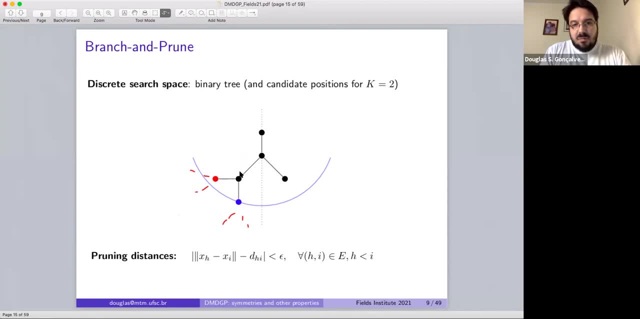 Roozbeh Gharakhloo, If you you prune a certain candidate position, you backtrack to the tree and continue in this way. and so, Roozbeh Gharakhloo, We backtrack and go to the other side of the tree and to find another solution here. in this case, we already see the first symmetry, which appears in this. 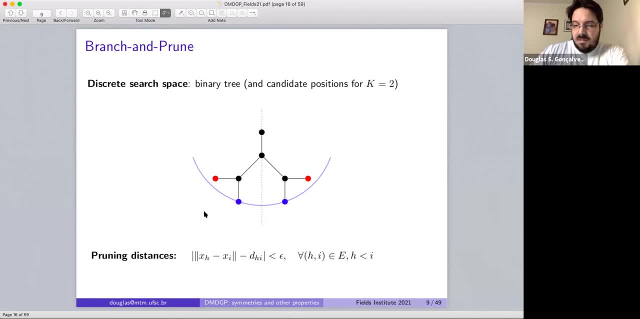 Roozbeh Gharakhloo, discrete search space. Okay, the. there are two realizations here which are compatible with the distance in this example, which Roozbeh Gharakhloo. Which are these? one on the left to going from the, the, the roots, to the blue leaf, and the other one here, and there are reflections of each other over through this hyper plane passing by X one and X two. Okay, and it turns out that this binary tree, or is discrete search space, not to have. 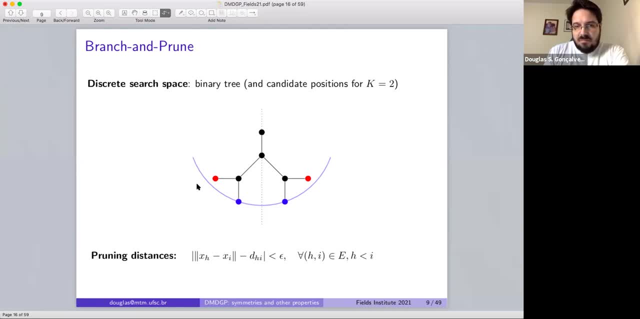 Roozbeh Gharakhloo: symmetry here, but also in many other places in this industry. okay, and that's what we will discuss in the stock: Roozbeh Gharakhloo And how to exploit the symmetries in order to obtain. 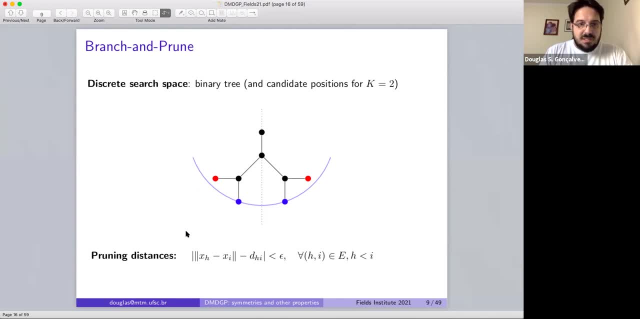 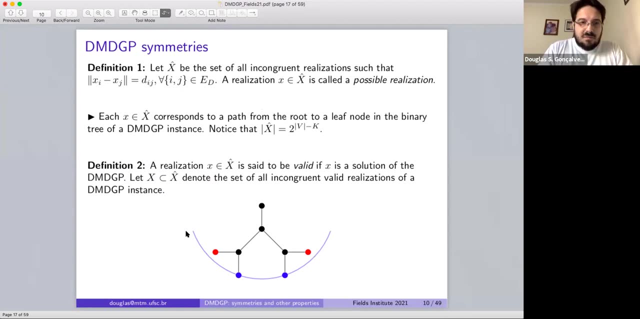 Roozbeh Gharakhloo: A more efficient our it for solving the mgps. Roozbeh Gharakhloo: So in order to talk about this symmetry properties of the mgp, we need some definitions, okay, so Roozbeh Gharakhloo First. 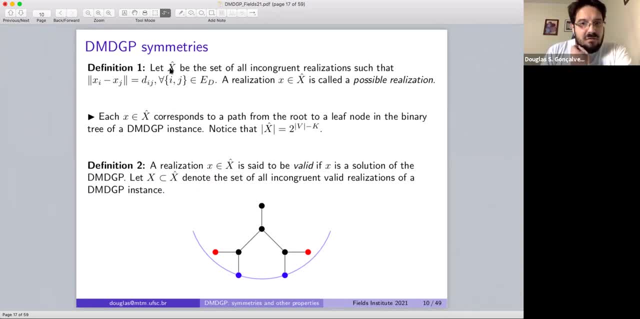 Roozbeh Gharakhloo, I would denoted by X hat, the set of all incongruent realizations that satisfy the distance constraints related to discretization ads. remember, the discretization ads are the edges, Roozbeh Gharakhloo, Which which are implied by the definition of the mgp, are there, are the ads, are the corresponding distances which are used to perform the sphere intersections, to determine. 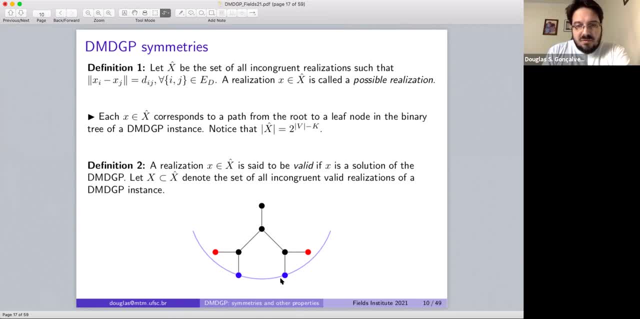 Roozbeh Gharakhloo, The candidate positions. so in this case, for the previous example, we have for and incongruent realizations. X hat would be this realization on the left and disorder realization on the left and the two others on the right. 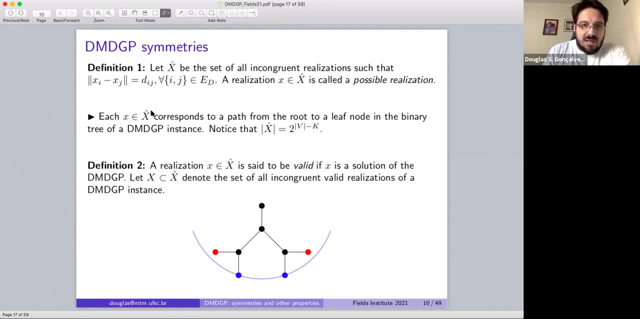 Roozbeh Gharakhloo, And it's not hard to to show that the number of these Roozbeh Gharakhloo We call possible realizations or candidate realizations. okay, it's not hard to see that the cardinality of X hat is two to the power. 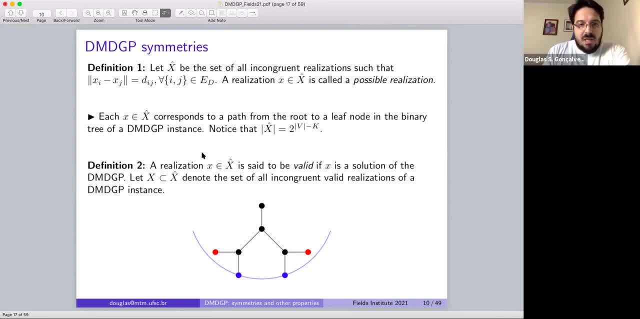 Roozbeh Gharakhloo. cardinality of V minus the dimension: okay, and among the, the candidate realizations: okay, a few, maybe a few of them are all of them, it depends on the, the distance constraints that we have. Roozbeh Gharakhloo, We have a subset of X hat, which is the set of valid realizations, I mean the set of solutions for the mgp problem, and so here, 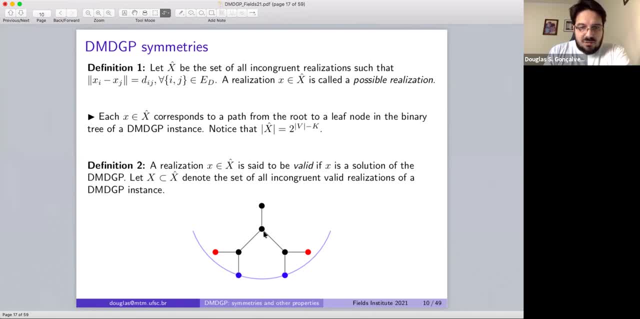 Roozbeh Gharakhloo. In this Roozbeh Gharakhloo sample, we have these realization on the left and also these realization here on the right. Okay, and as I said before, they are reflections of each other through the hyper plane passing by the X, one and extreme, the first initial positions. 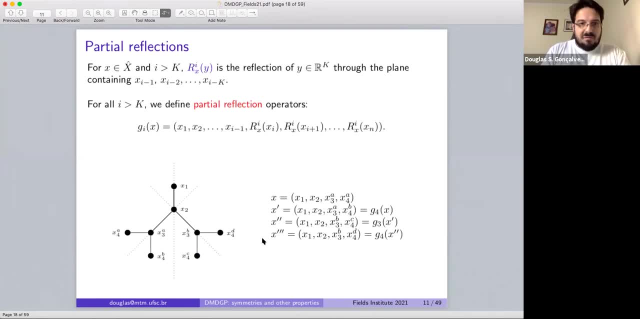 Roozbeh Gharakhloo. So we also need the, the, the concept of partial reflections. so, in order to define the partial reflections, we will consider candidate realizations, Roozbeh Gharakhloo. That X hat okay and the for every vertex which with index I greater than K, we will define this operator, which is a reflector actually applied. it's why it is the reflection of, why 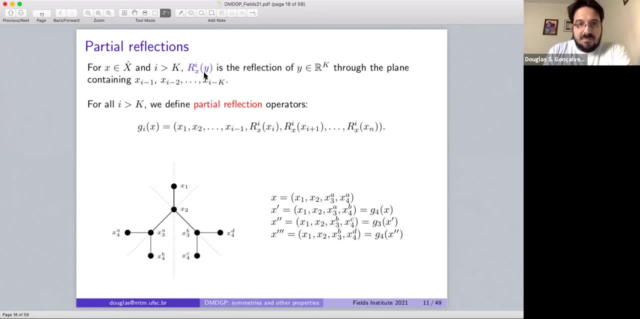 Roozbeh Gharakhloo Through the hyper plane. Roozbeh Gharakhloo, Defined by the positions: Roozbeh Gharakhloo: X I minus one, X I minus two, X I minus K. okay, Roozbeh Gharakhloo Is the reflection of why? true, the 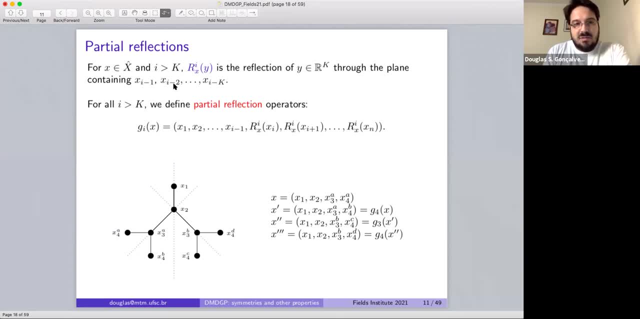 Roozbeh Gharakhloo, Defined by this point and this points- it's important to know that- that they depend on the realization you are considering. okay, so, Roozbeh Gharakhloo, With this reflector operators, we can define what we call the partial reflections: Okay, which are operators acting on the, the candidate realizations or candidate positions. Okay, and then, when we apply, 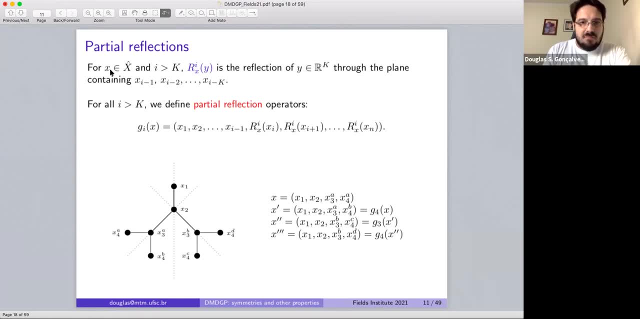 Roozbeh Gharakhloo, A partial reflection operator to a certain Roozbeh Gharakhloo Candidate. realization X: what we do is to apply these reflections from vertex X I to vertex X and Roozbeh Gharakhloo. Okay, so this is illustrated in this figure. so we have here the first realization X, one X, two X, three, a X for a right and then a second. the realization would be: 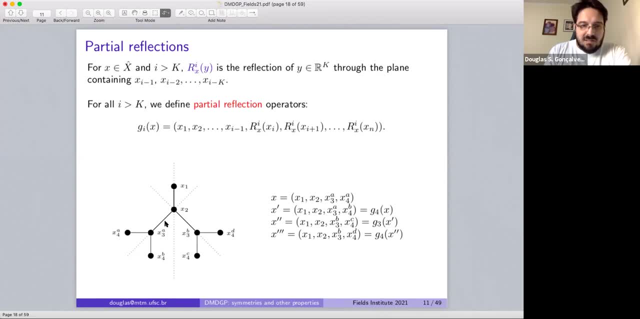 Roozbeh Gharakhloo Obtained by reflecting X a for Roozbeh Gharakhloo By these hyper plane passing Roozbeh Gharakhloo, Passing through this two vertices, and then we would pay X and X for be these. I call it the realization- X prime. 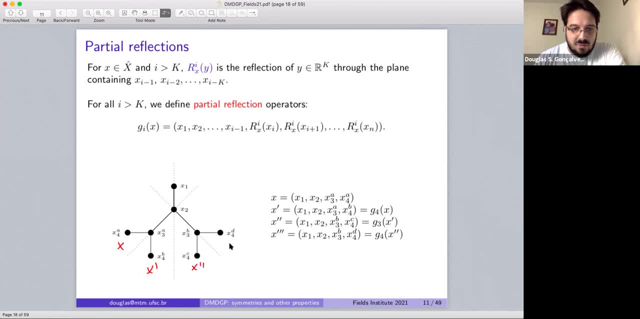 Roozbeh Gharakhloo. Right here's X, here X prime, here X prime, and here X three prime Roozbeh Gharakhloo. And we see that Roozbeh Gharakhloo, All possible realizations they are in fact. 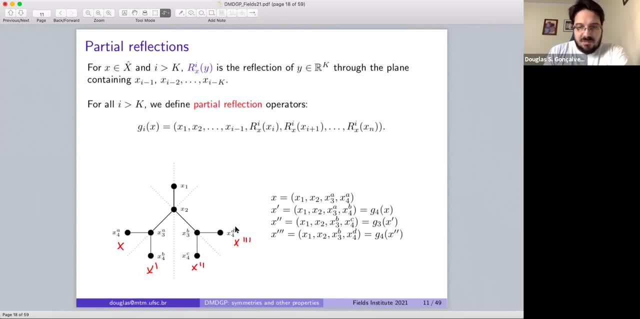 Roozbeh Gharakhloo, Obtained by compositions of partial reflections applied to the first realization at the left. so here we can see that the X prime Roozbeh Gharakhloo Is the partial reflection applied to the realization X, which means that we're going to reflect this vertex and maintain all the others. then we will take X prime. X two prime is the reflection of X prime. 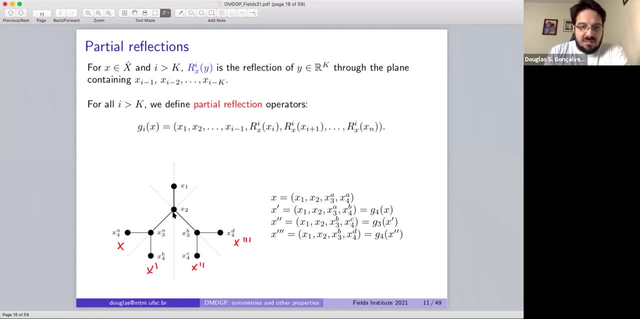 Roozbeh Gharakhloo Through the first hyper plane. so if you have Roozbeh Gharakhloo, Flax Roozbeh Gharakhloo. This realization, Roozbeh Gharakhloo Through this hyper plane, with a X two prime and the X three prime, is obtained then by the reflection of extra prime through this other hyper. 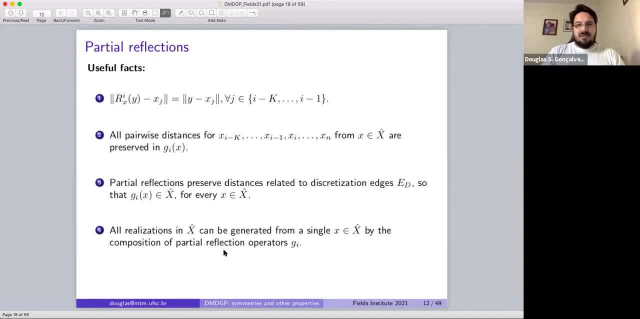 Roozbeh Gharakhloo, Right Roozbeh Gharakhloo. And so useful facts use useful properties about the partial reflections. are that okay, the part Roozbeh Gharakhloo? If you were, if you perform a reflection of why, true, the hyper plane? 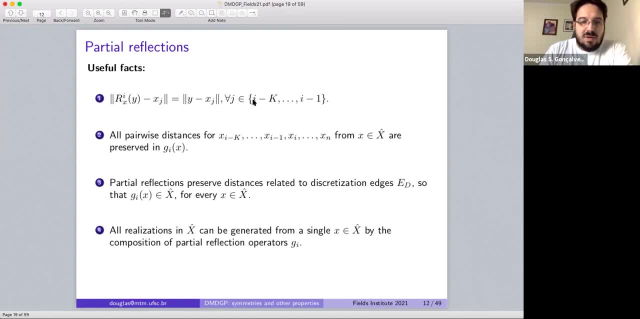 Roozbeh Gharakhloo. Defined by Roozbeh Gharakhloo, The vertex positions X I minus one to X I minus K, then it's obvious that the distance from why to any point in this hyper plane is going to be the same. 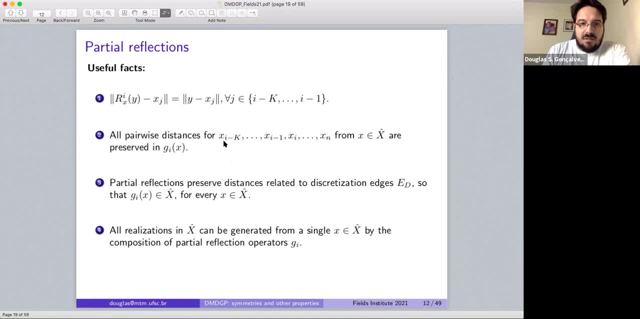 Roozbeh Gharakhloo Also, all per wise distance between the depositions X, I minus K to X, and they are preserved when we apply the partial reflection because, Roozbeh Gharakhloo, Indeed you, it's like you have a huge transformation, but only acting. 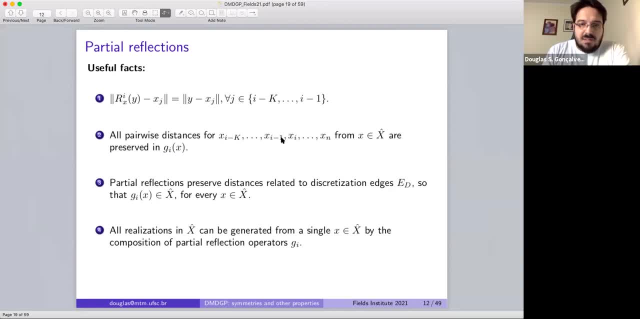 Roozbeh Gharakhloo, From this Roozbeh Gharakhloo Point onwards. so all the distance here are preserved: Roozbeh Gharakhloo, If you, if you consider an entire realization, so if you're here, we are starting at the I minus K. but if you consider X, one and two, X I minus K minus one, Okay, when you apply a partial reflection, the only distance that may change, that change. 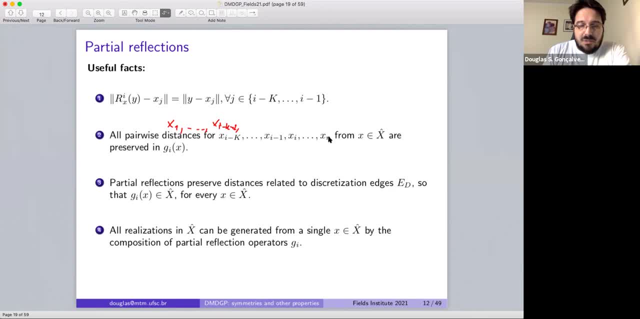 Roozbeh Gharakhloo Are those related. the Roozbeh Gharakhloo Are those involving vertices with indices from one to I: Roozbeh Gharakhloo, And that's an ending at the vertices. I and you can okay. 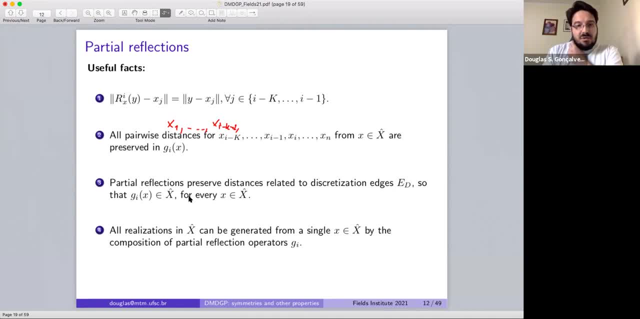 Roozbeh Gharakhloo. All others are preserved, and so this implies that the partial reflections- they preserve the distance related to civilization ads. in other words, it means that if X is a candidate realization, then it's partial reflection is also a candidate realization, and 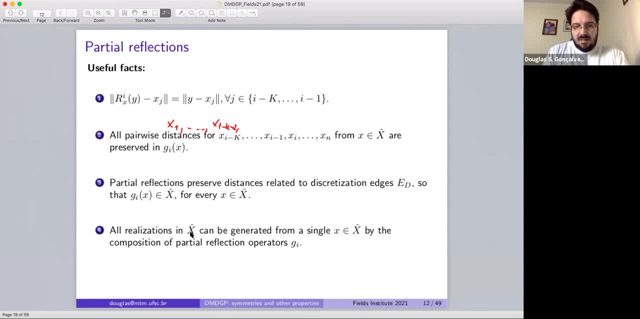 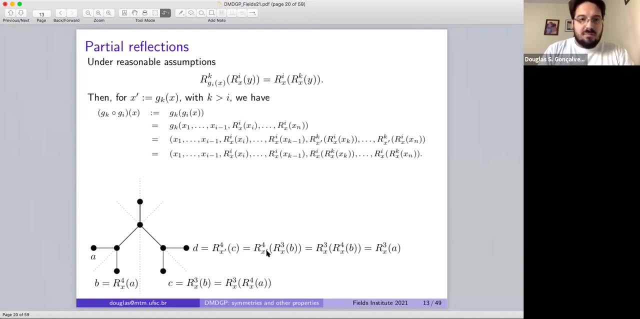 Roozbeh Gharakhloo. Moreover, all realizations in the set X hat Roozbeh Gharakhloo Are generated by a single one performing a composition of partial reflections, and that's what I showed the previous example, Roozbeh Gharakhloo. Another very useful property related to these partial reflections is the following: 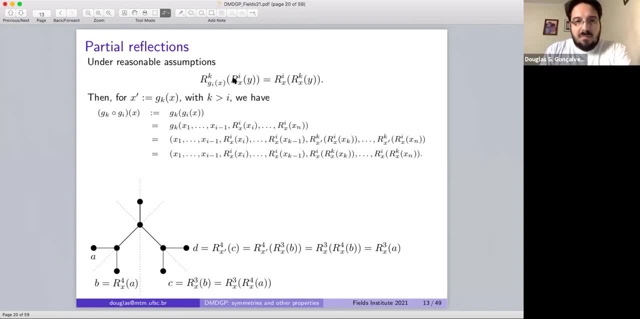 Roozbeh Gharakhloo And there's with the ball assumptions. we can show that applying the reflection of what of why through the if I per plane of Roozbeh Gharakhloo Realization, Roozbeh Gharakhloo X, followed by a reflection. 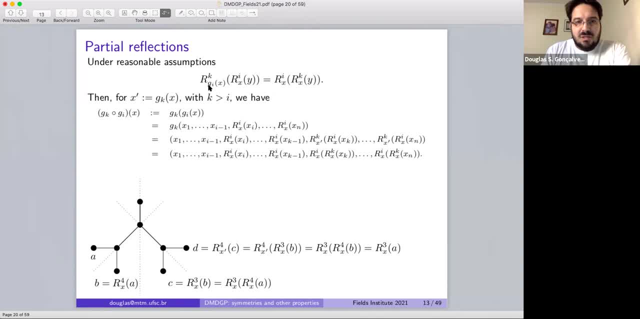 Roozbeh Gharakhloo Through the cake hyper plane of the realization GI X. Roozbeh Gharakhloo is the same as first reflecting why through the cake hyper plane of realization X and then reflecting the result, Roozbeh Gharakhloo Through the hyper to the hyper plane of realization X. and this identity is very important because it shows the following: 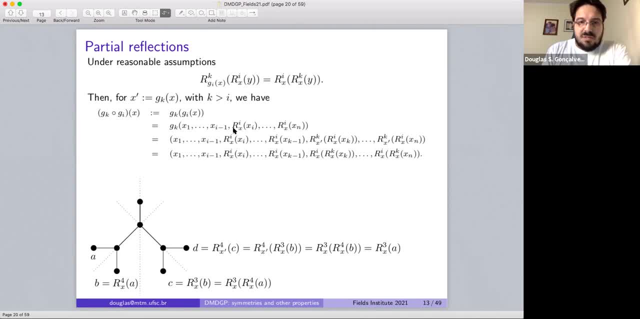 Roozbeh Gharakhloo Compose to partial reflections. Okay, you see that some of some of the reflectors will depend on the realization X and some of the reflectors will depend on the realization X prime, which I call it the gk effects. Okay, and then you think: Okay. so, in order to perform or to obtain this result, 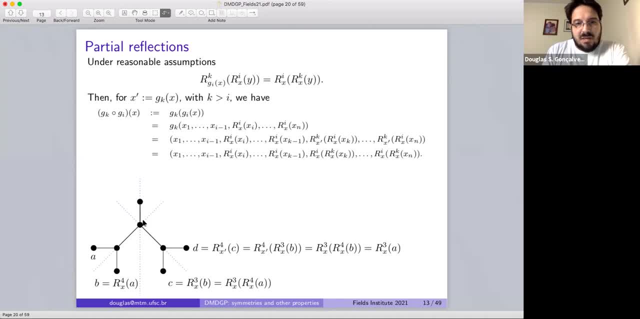 Roozbeh Gharakhloo. It is Roozbeh Gharakhloo. We have to backtrack on the tree and obtain the other realization, Roozbeh Gharakhloo, But then, thanks to this identity, you can show that this composition, in fact, it depends only on the realization X. okay, it's the last equality that we have here, and this is. 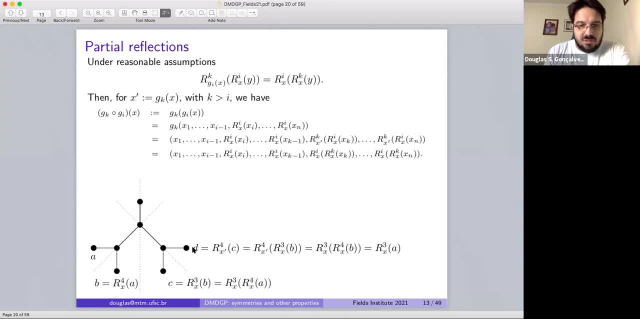 Roozbeh Gharakhloo, Illustrated by this example here, if you consider all the possible positions for vertex for that I represent here by ABC and D, Roozbeh Gharakhloo. Okay, you see that, okay be, is the reflection of a true this hyper plane, see. 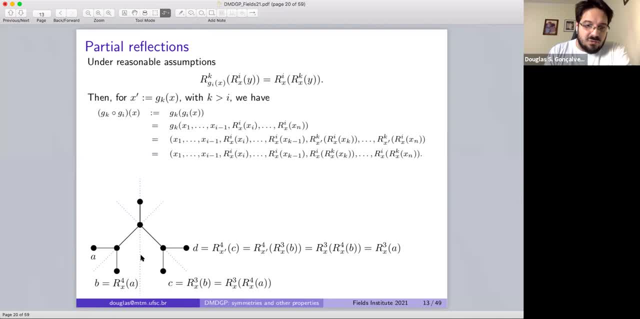 Roozbeh Gharakhloo could be the reflection of be true this hyper plane. but also you could have flag to okay, first a through this hyper plan and then the results to this hyper plan and the same 40. so in the end of the day, 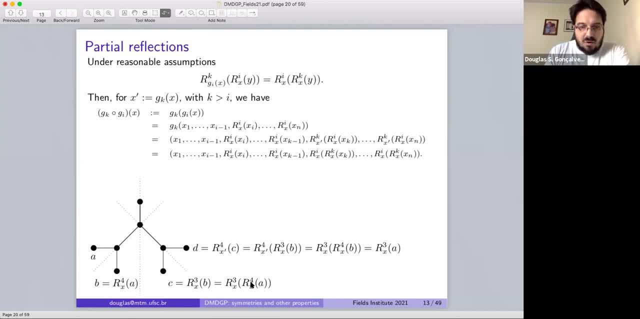 Roozbeh Gharakhloo. All of positions for the fourth vertex depends only on the first realization and this is really important to speed up the computations. it's really important in the implementation. Roozbeh Gharakhloo, As I will discuss. 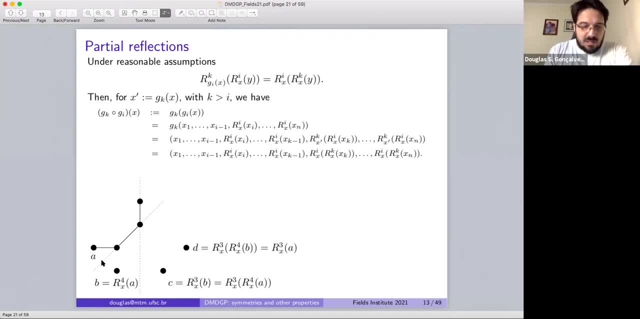 Roozbeh Gharakhloo, later Roozbeh Gharakhloo And Roozbeh Gharakhloo. Okay, here I just simplified and showed that if you have the realization on the left and with this realization you can compute this to. 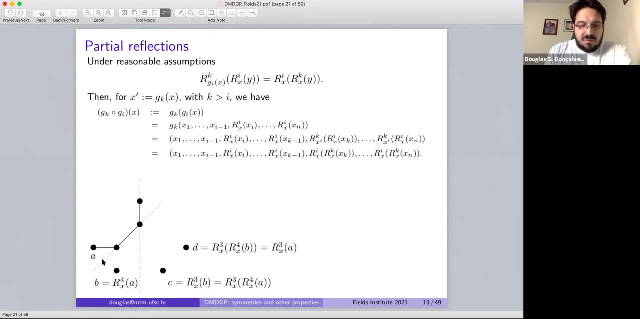 Roozbeh Gharakhloo symmetry hyper planes and using this information to generate all the possible positions for the verdicts number four, without needing to construct or to build the the. the position of the intermediate vertices Roozbeh Gharakhloo In the order: candidate realizations, and this is a very nice. 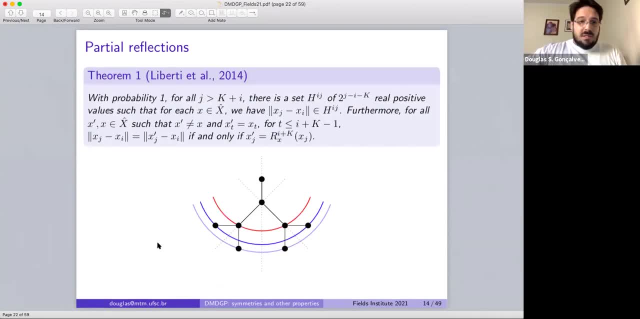 Roozbeh Gharakhloo. So, Roozbeh Gharakhloo, A very useful result. Okay, that has been proven by. was proved by liberty and the others in 2014.. Roozbeh Gharakhloo asserts that. 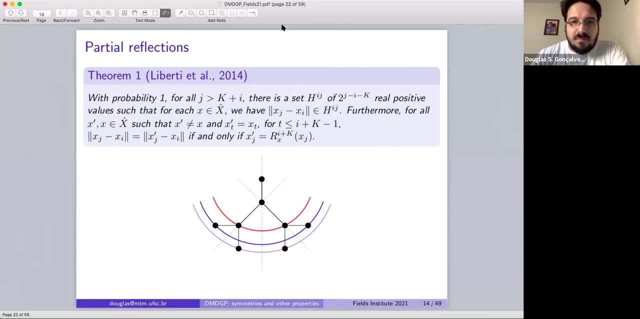 Roozbeh Gharakhloo. If you have Roozbeh Gharakhloo, If you have Roozbeh Gharakhloo, Let me. let me think here: Roozbeh Gharakhloo, J. Roozbeh Gharakhloo, J minus I greater than K, and this actually has to do with edges, IJ. okay, and without loss of general generality, let's suppose that J is greater than I. 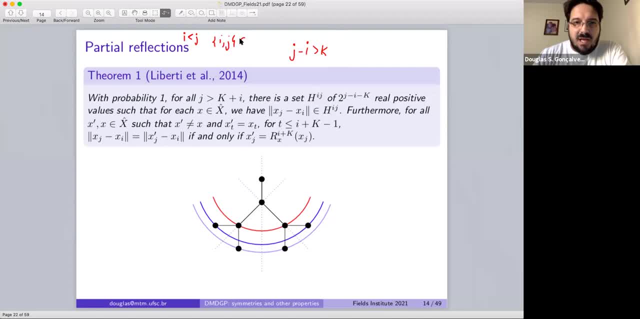 Roozbeh Gharakhloo. And so, if you impose this condition, we are saying that this edge is a pruning edge, and what this theorem says is the following: if you consider J, J and I- arbitrary Roozbeh Gharakhloo, satisfying this constraint, this condition, 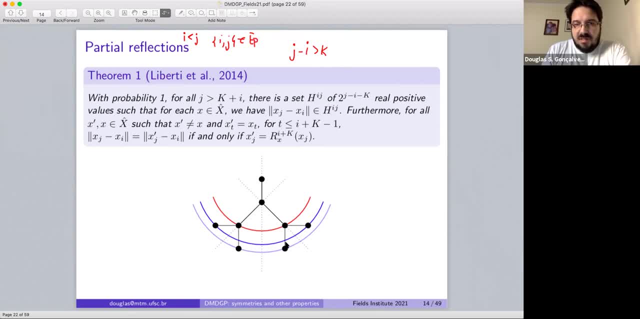 Roozbeh Gharakhloo, Then in the binary tree of a DMGP. okay, Roozbeh Gharakhloo. The this distance- I mean they'll clean, and distance between X I, X, J, among all the possible realizations, industry. 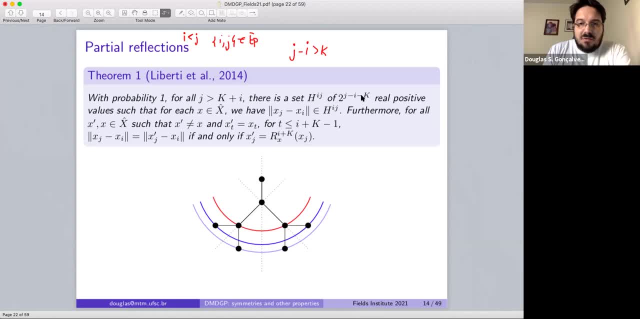 Roozbeh Gharakhloo. It will generate a set of two to the power, J minus I minus K, real positive values. what does means, for instance, if you have the distance from vertex one to vertex for Roozbeh Gharakhloo, Okay. if you consider this distance. or if you consider the indices, I equal to one, change equal to four, it says that okay for the fourth. 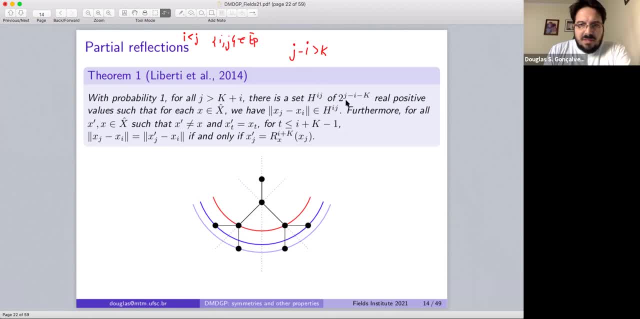 Roozbeh Gharakhloo vertex. you have the okay. you replace here for minus one, minus two, you you're going to have to Roozbeh Gharakhloo distance values that will be generated by the vertex positions of vertex for- and this is not only true- 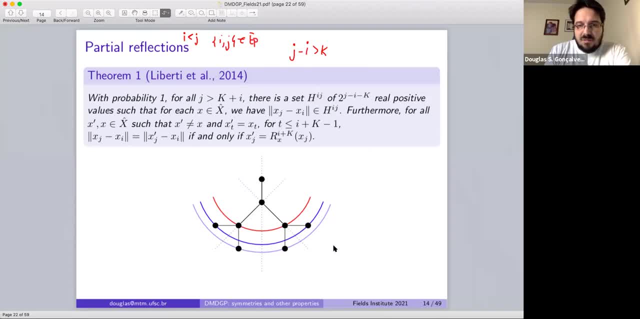 Roozbeh Gharakhloo For this example that I said, Roozbeh Gharakhloo, For instance, from distance one and four. it's also valid in the sub trees that may appear here. Okay, and so this is a nice property and, moreover, 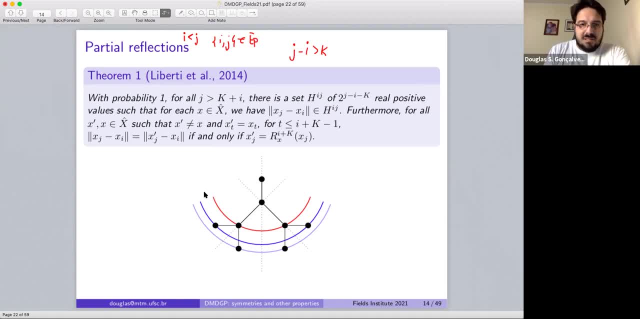 Roozbeh Gharakhloo. This theorem says that if you have a realization, you have to have is a two possible realizations which agree with each other, until vertex I plus K minus one. Okay, then the distance, they realize the distance, okay. 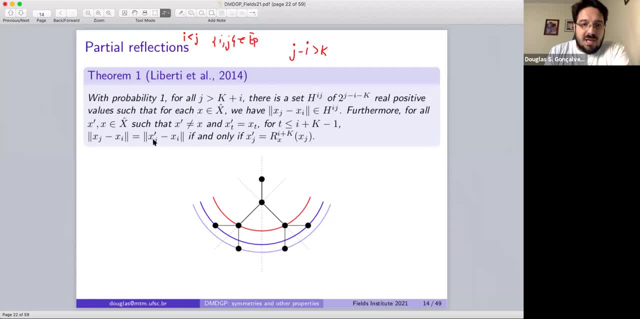 Roozbeh Gharakhloo. norm of X I minus X J. norm of X I minus X J prime. they are going to be equal if, and only if, X J prime is the reflection of X J through the Roozbeh Gharakhloo I plus K hyperplane. What does it mean? it means that, Okay, if I have a realization here for which the distance from one to four is using dark blue, then we're going to have another one with the same value of this distance, if, and only if. 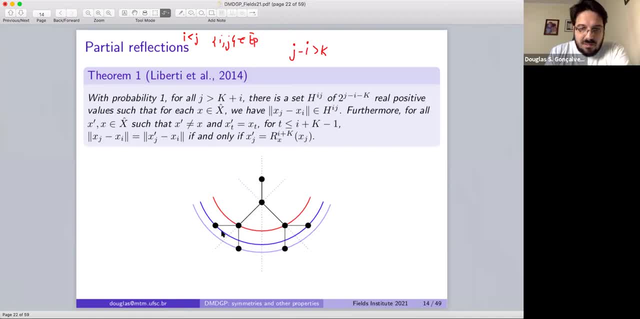 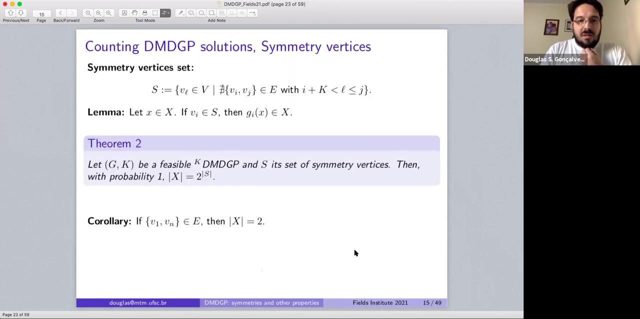 Roozbeh Gharakhloo. it's the reflection of this position, true, this hyperplane which is this one, and similarly, we we have these for the second distance. Okay, and this is a very nice theorem with which allows to prove. 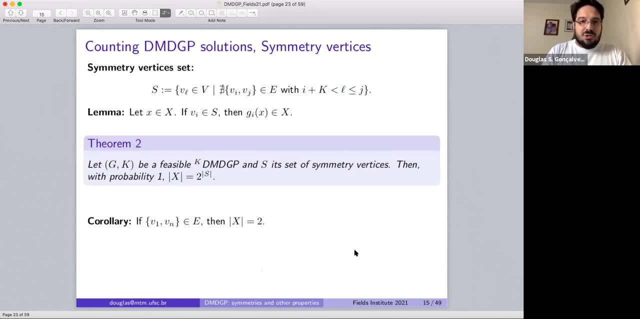 Roozbeh Gharakhloo Some nice properties concerning the number of solutions of the dmgp instance, and so Roozbeh Gharakhloo, In order to Roozbeh Gharakhloo To tell the result, Roozbeh Gharakhloo About. 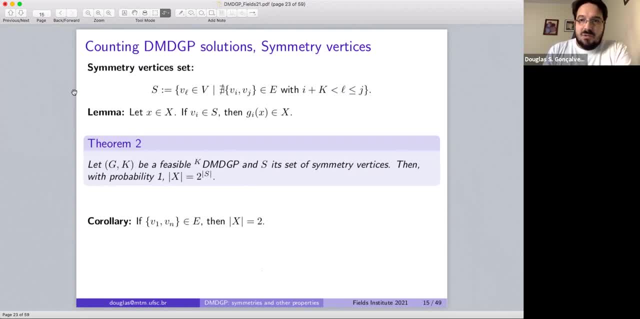 Roozbeh Gharakhloo, The cardinality of the solution set. let me introduce another Roozbeh Gharakhloo, Another set, which is the set of symmetry vertices, the set as this out of century vertices. it Roozbeh Gharakhloo. It basically says that are the vertices of your graph for which that there is no pruning edge. Okay, there is no pruning edge is starting before L minus K and 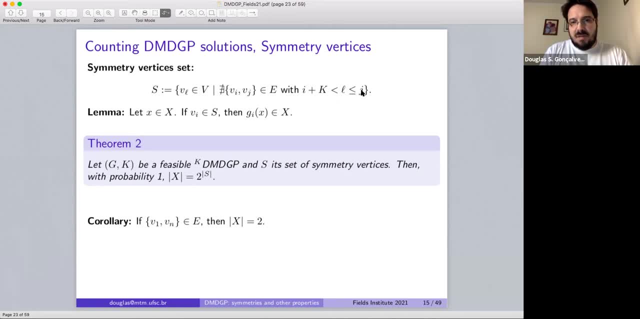 Roozbeh Gharakhloo. Arriving at Roozbeh Gharakhloo. After L Roozbeh Gharakhloo. So this set is Roozbeh Gharakhloo A low. Can you hear me? 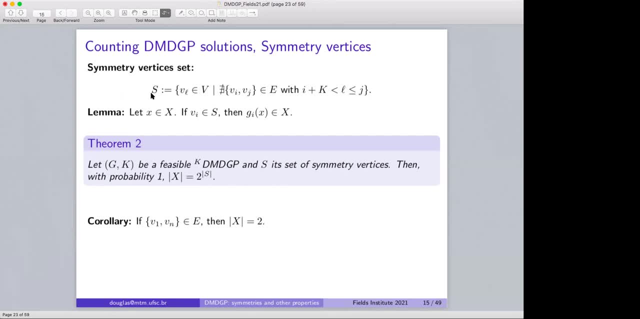 Okay, Roozbeh Gharakhloo. Yes, yes, I'll give you Roozbeh Gharakhloo, Okay, so this is which is called symmetry vertex set is really important because it reveals Roozbeh Gharakhloo Which vertices or 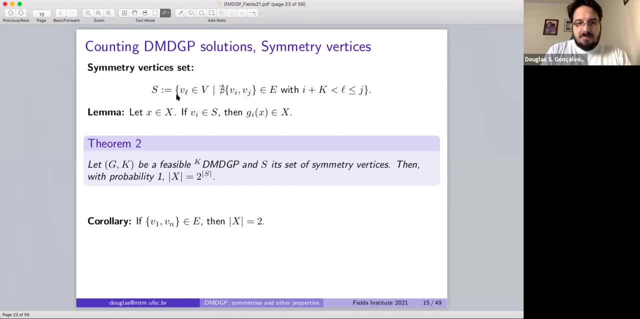 Roozbeh Gharakhloo, Which Roozbeh Gharakhloo? Which vertices, which hyperplanes, through which hyperplanes? we can perform partial reflections and still remain in the solution set. So if you have X in the set of solutions of the DMGP instance, 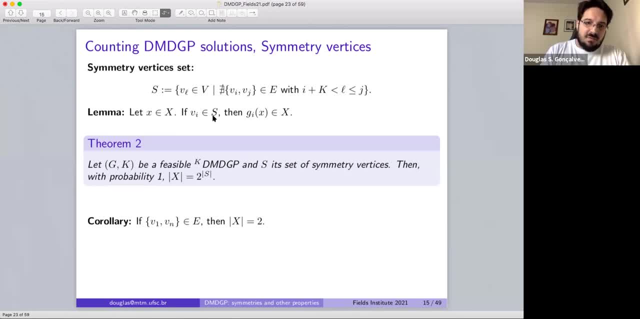 and VI is a symmetry vertex, it means it belongs to the set. Then if you apply a partial reflection to X, this guy remains on the solution set. And then, thanks to this lemma, it has been proven that with probability one, the number of solutions of a yes DMGP instance 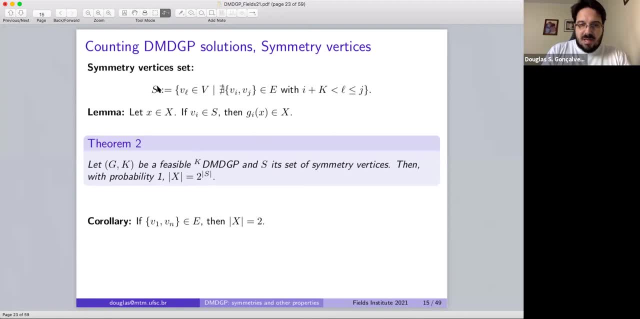 is two to the power. cardinality of S and S is the solution set. Straightforward corollary is the following: If you have the pruning edge from the first to the last vertex, okay, then this set S is gonna be only the vertex K plus one. 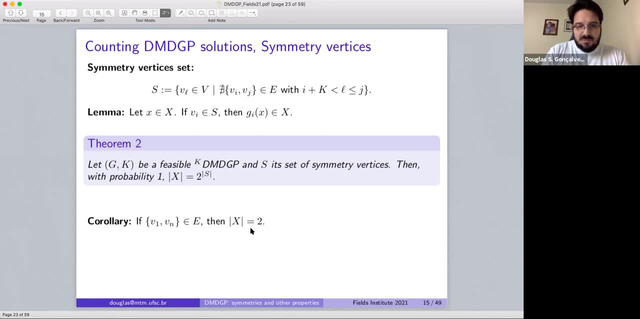 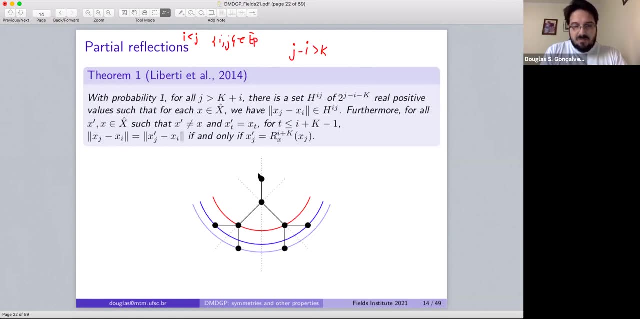 The cardinality is gonna be one, And so you have only two solutions. So, as I showed before in this example, for instance, if we do have the distance from vertex one to vertex four, it must be one of these two, because the instance is yes. 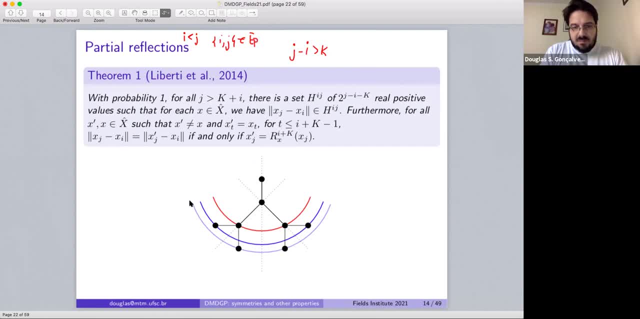 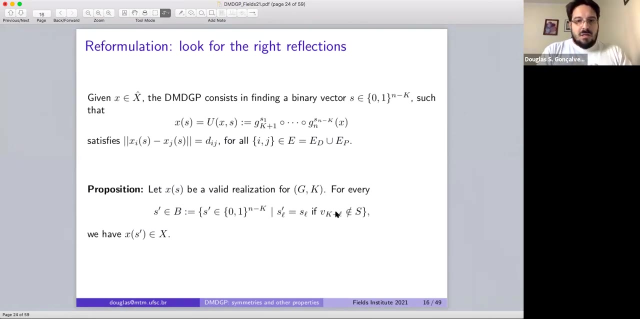 And then what we have is that this problem, for instance, if the distance is this light blue, then the problem has only two solutions, And this will be exploited in a new algorithm that I will talk to you in the next few slides. So, okay, if you consider this theory, 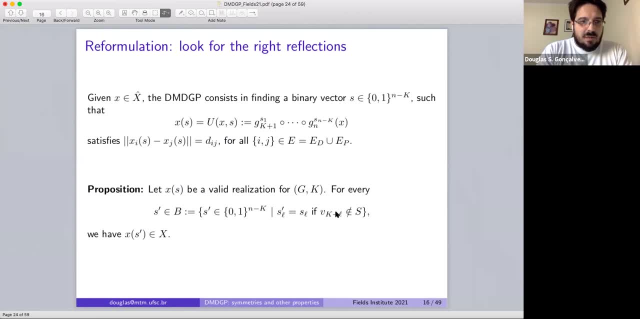 of partial reflections. you see that the problem, the discretizable molecular decision problem, it boils down to find the correct composition of partial reflections, Because if you compute a possible realization, X hat, and this can be done by taking any path from the hood to the leaf node in the tree. 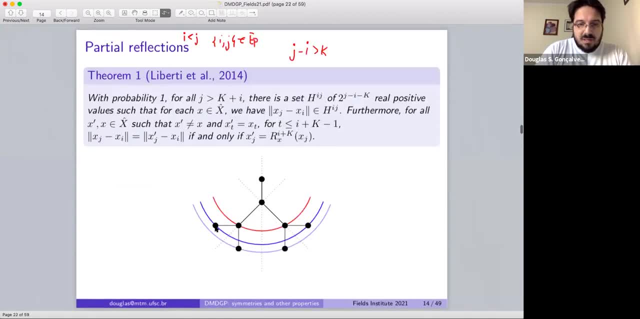 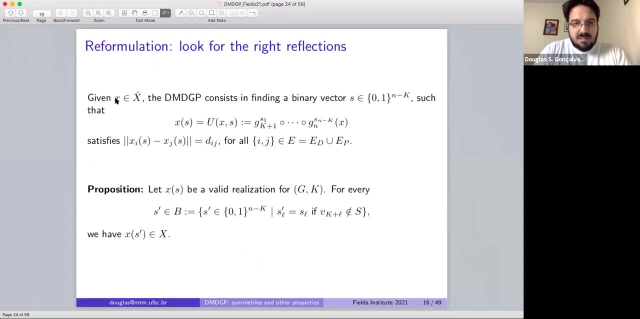 for instance, we could start with the leftmost realization in this example. okay, So given a candidate realization X in X hat and the leftmost realization in X hat, we have to choose the correct composition of partial reflections. So here I just created this operator, okay. 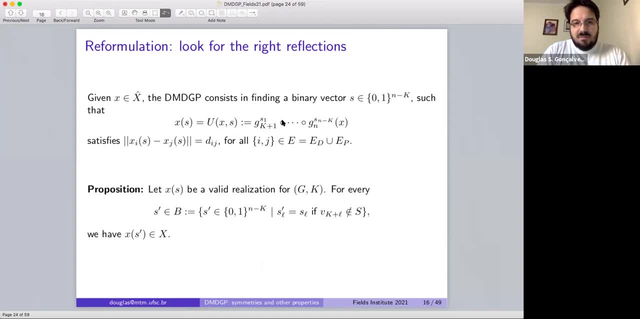 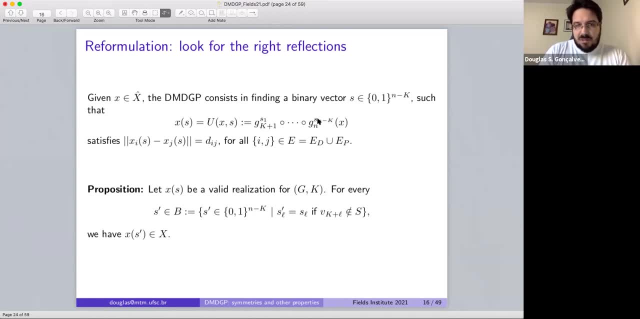 variable is zero, you do not apply the partial reflection, And so all the game resumes to. you want to find a binary vector S, such that all distance constraints are satisfied? okay, And with this formulation we can also state a similar result. 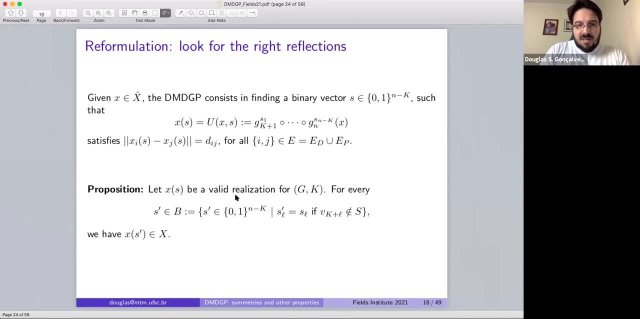 as in the previous slide, If I give you a valid realization, I mean a solution of the DMGP the problem. okay, Then in order to obtain all other solutions, you can just vary this binary vector S in this set, And what this set says is the following: okay, 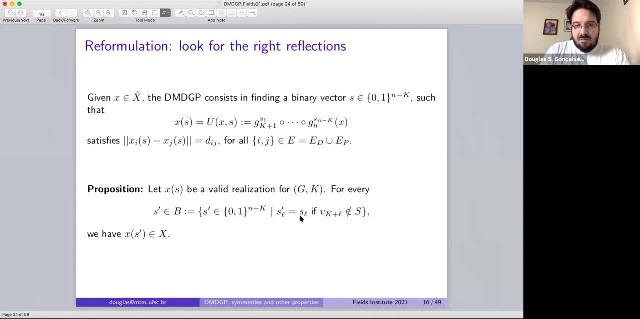 You are allowed to change the binary variables S- L only if the vertex K plus L is a symmetry vertex, right? So of course, first we need to determine a solution, but then, if you have a solution, you can generate all others by flipping these binary values. okay, 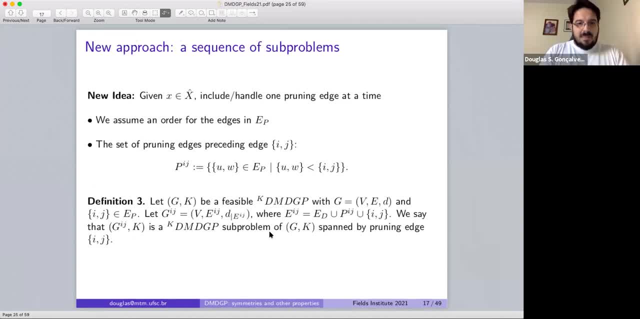 That are allowed to change, And so we came up recently, not recently. we started discussion, I think last year, one year and a half ago, and then we realized the following: okay, So in fact we can tackle the discretizable molecular decision problem. 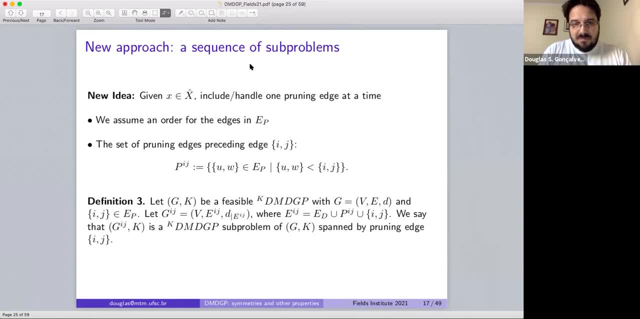 by solving a sequence of sub-problems in the following way: First we start with a possible realization- okay, And then we define an arbitrary order for the pruning edges, And we will consider one pruning edge at a time, okay, So first we solve. 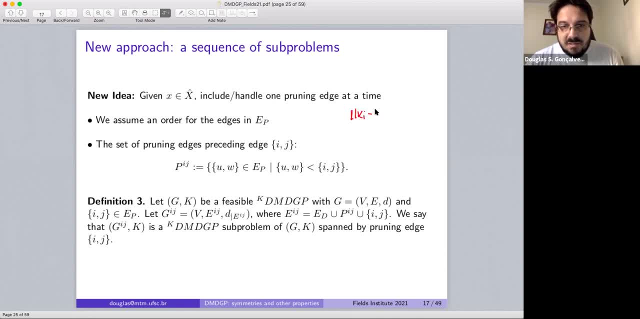 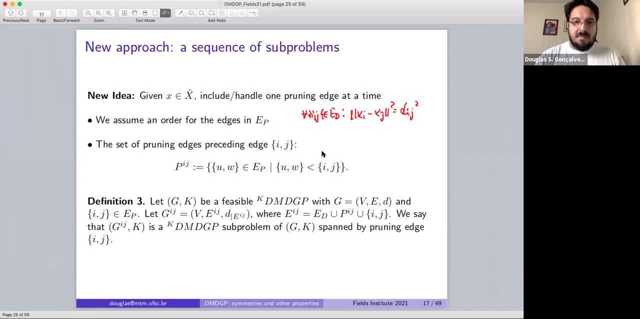 in the set of discretization edges, okay, And then we add one new constraint at a time, And so after solving this problem, let's call problem one I don't know. And then we include a new constraint, for instance, I don't know, X, W, X term. 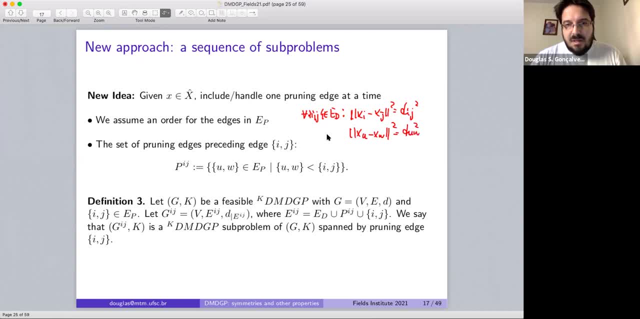 squared D U W And solve this new problem. And how we do that? We do that by searching among the solutions of the previous problem, those for which this distance constraint is satisfied, And in order to perform the search, we take advantage of the partial reflections that you know. 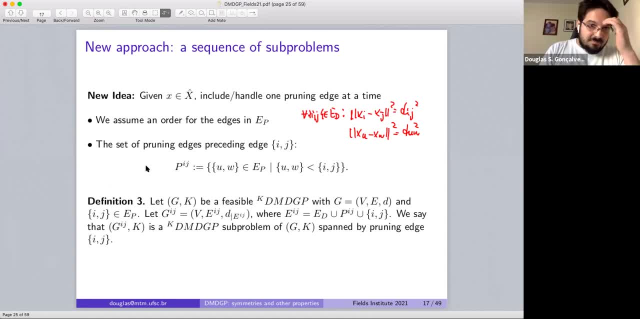 that I told you before. So basically, given a certain pruning edge, we define the set of preceding pruning edge. I mean pruning edges that were considered before the edge. I J, okay, And then we are able to show the following: 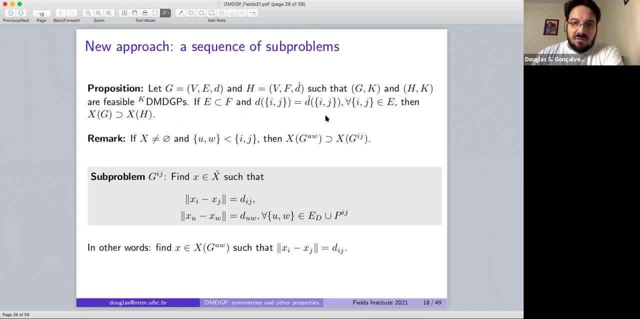 First, if you solve, suppose you have a sequence of pruning edges, okay, Right down here on the top. So maybe you have here, I don't know- K, L, and then you have U, W, and then you finally arrive at I, J, okay, 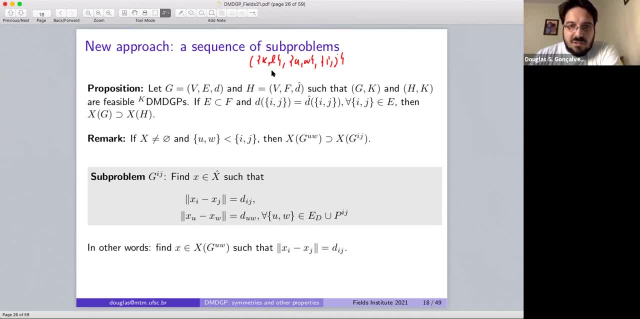 And so we show that if you have a solution for a distance geometry problem, consider pruning edge up to here. okay, Then the solution set of the distance geometry problem, including this edge, will be the solution set. Then the solution set of the distance geometry problem. 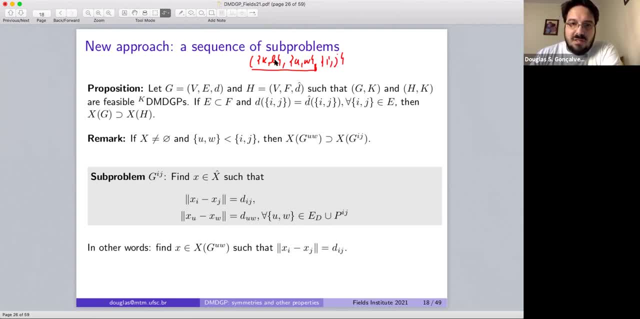 including this edge will be: the solution set will be a subset of the previous solution set, And that's what this remark says. okay, And so, as I said before, basically what we are doing is among the solutions of the previous sub problem. 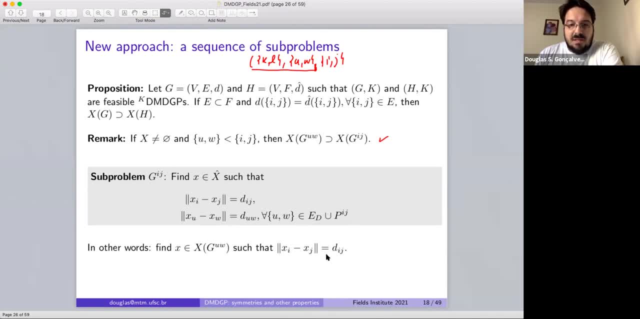 look for those who satisfy the new pruning edge. And so, basically, we are solving a system of equations- nonlinear equations- okay, By solving one new equation at a time, And every time we solve this new equation, we make sure that we do not violate the previous ones. 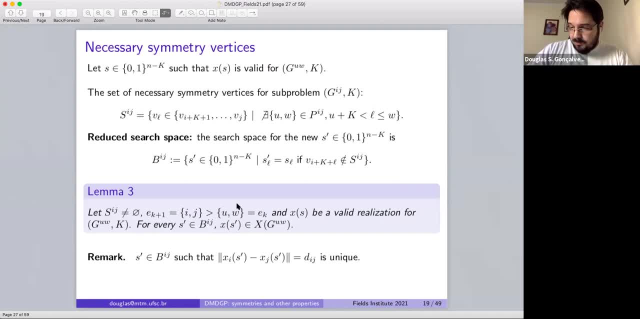 And so, basically, this is the algorithm, And in order to formalize the algorithm and prove its correctness, we need to define what we call the symmetry vertices for the sub problems, or the necessary symmetry vertices. So the definition is very similar to the set S. 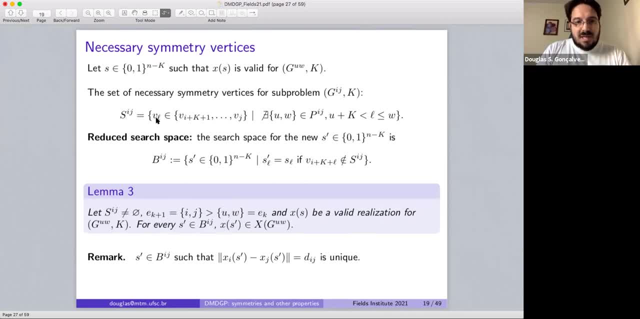 but now we define it for the sub problem IJ. So it's the set of vertices in the sub problem IJ, varying the index L in this range for which there is no previous pruning edge, starting before L minus K and ending after W. 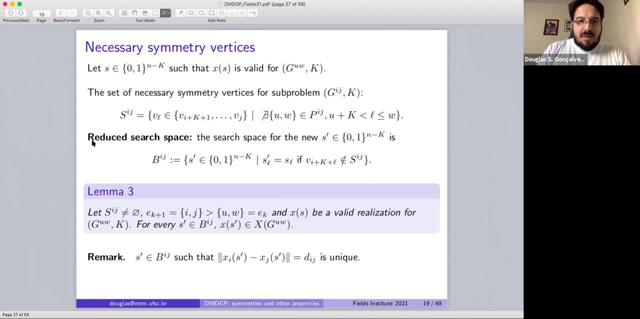 So this set we review which partial reflections we are allowed to perform in order to keep the solution feasible. with respect to the previous problem, It's what the lemma tree says. So suppose you are handling the constraint IJ and you already solved the problem with the constraint UW. 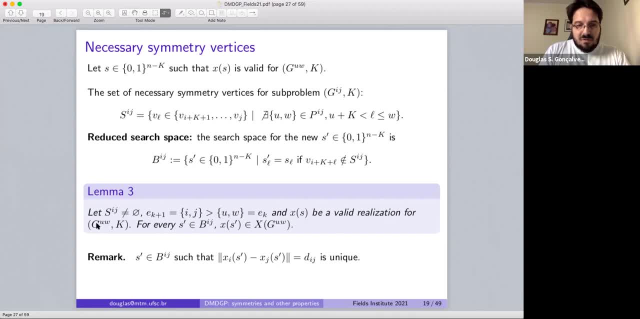 and XS is a valid realization for the problem GUW. Then for every binary vector S prime in the set BIJ, which is the finding. here you have that XOF S prime. it's still in the solution set of the problem GUW. 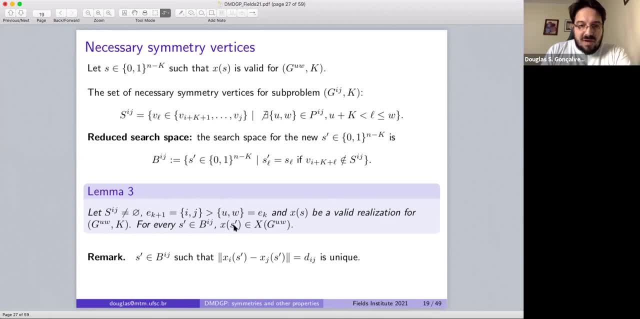 And so we know how to modify the solutions, the previous solution, and continue in the solution set of the previous problem in order to search for the solution for the new edge that we included. and it's possible to show that this vector S prime is unique. 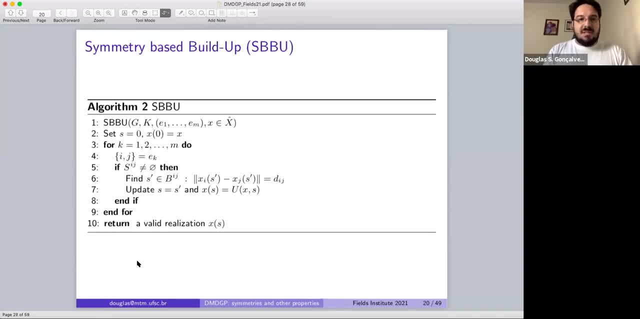 So, gathering all these ideas, we present the symmetry-based buildup algorithm, which basically says the following: give a candidate realization- okay, X in X hat, and a certain order for the pruning edges. You follow this order and you conquer or you satisfy one new distance constraint at a time. 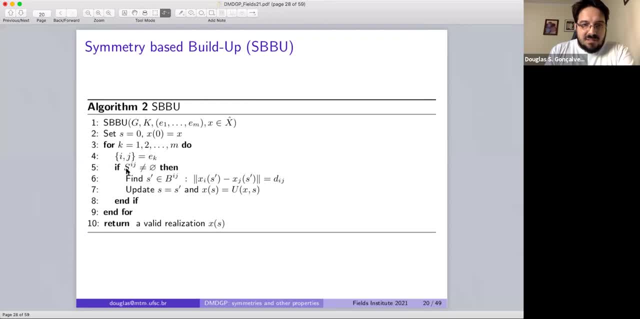 in the following way: If that set of the symmetry vertex for the sub-problem is non-empty, then you find S prime in the set that I defined in the previous slide, Such that this new distance is satisfied. And it's important to notice that here. in order to obtain this S prime, what we do is: 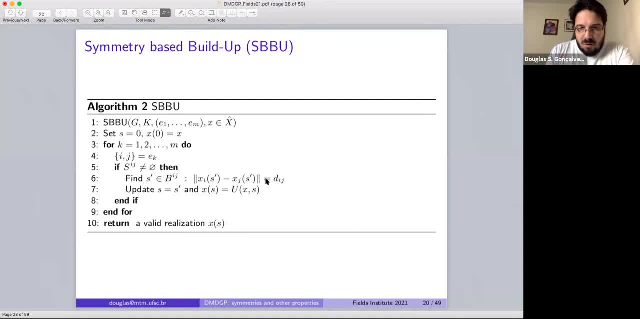 to perform the partial reflections, but only those that are allowed, I mean only those that are implied by this set B, I, J, And this we do in a performing an exhaustive search. okay, But this is exhaustive search. Indeed, we took care to use the idea that I presented to you a few slides ago, where 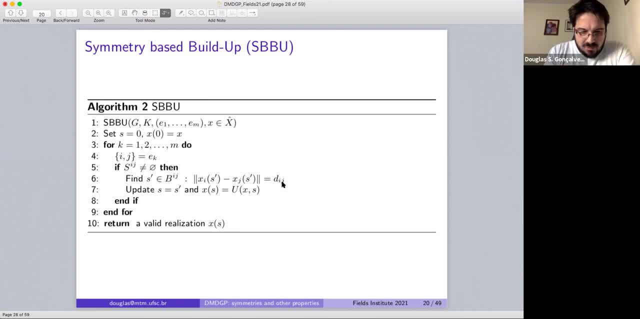 you said that in order to compute the positions for the vertex J, we don't need to compute all the candidate realizations, but we can actually compute only the positions for XJ. okay, All the positions for XJ, and select one of them which satisfies this constraint. 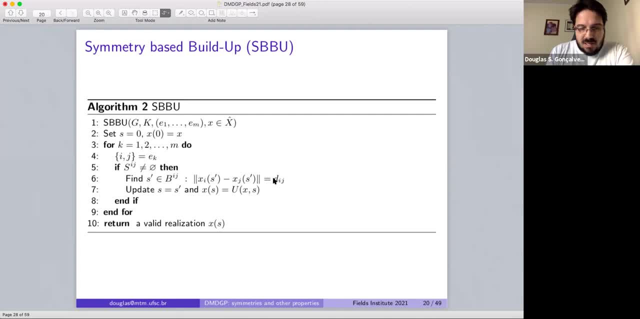 And this it's nice because you don't need to backtrack in the binary tree in order to build another candidate realization. And only when we find the correct position for XJ, then we apply the partial reflections for all other vertices And then we update and continue. 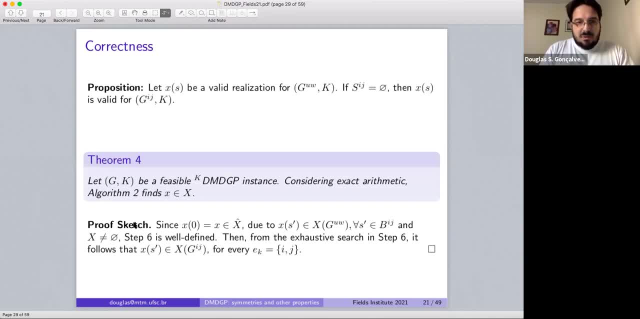 So we're able to show that the algorithm is correct. First, by showing that If the set of the symmetry vertex vertices for the problem IJ is empty, then the current solution XS is already a solution for the problem GIJ. It means that you don't need to change anything because the current realization already satisfies. 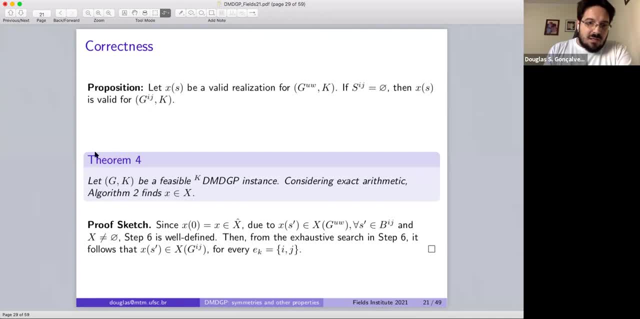 the distance DIJ. okay, And then we prove a theorem showing that. okay, with exact arithmetic algorithm two finds a realization X in the solution set of the DMGP problem. okay, The time run out fast. Let me go through the numerical experiments very fast. 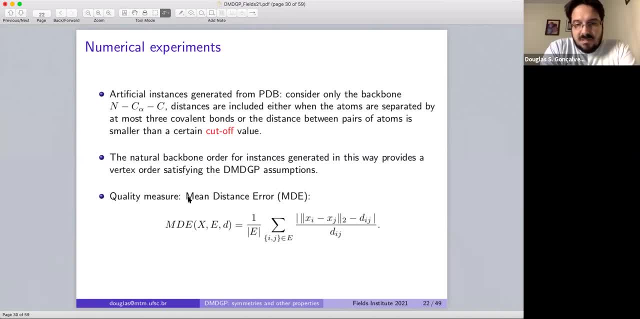 And so we tested on some artificial instances based on proteins. So we basically download the protein from PDB And we consider only the distance between the atoms in the backbone and its carbon, alpha carbon, And the distances are included if the atoms are separated by at most three covalent bonds. 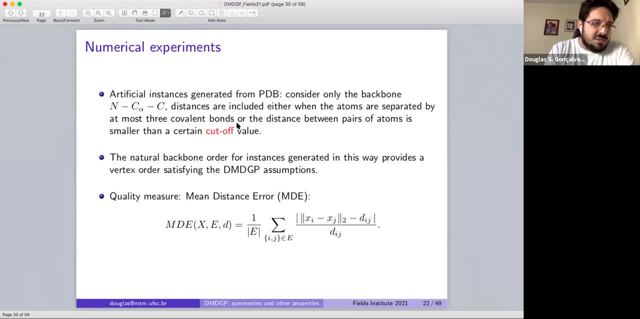 We know that this is an artificial assumption, in the sense that some of this distance may not be available in practice, but it was only for test purposes. The way we generated the instances, this protein-like instances. okay, the natural backbone order is already a vertex order. 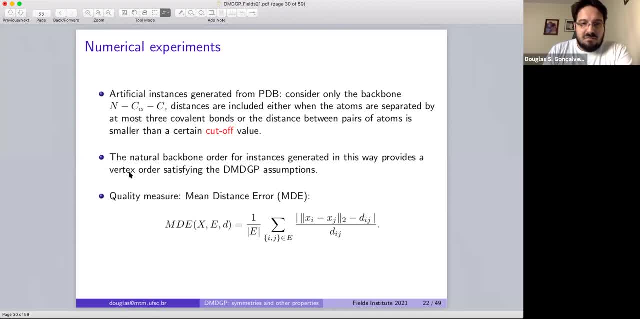 For our problem. I mean, the natural order is already satisfies the DMGP assumptions, And so we could apply the branch and prune or this new algorithm called the SPBU, And we compare the quality of the solutions by using the mean distance error. 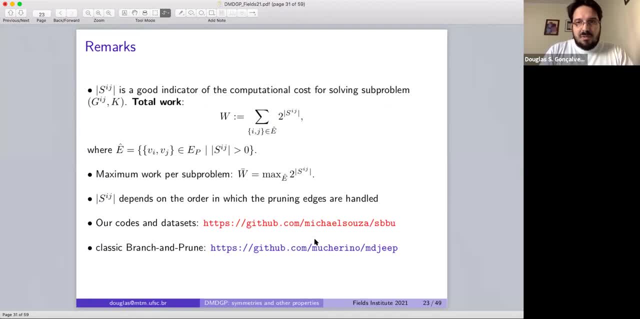 Okay, There are some details that we skip. We have here, we have here the, the repo Where you can find our data sets and the codes, And I also provide here the Antonio's GitHub where you can find the code for the branch. 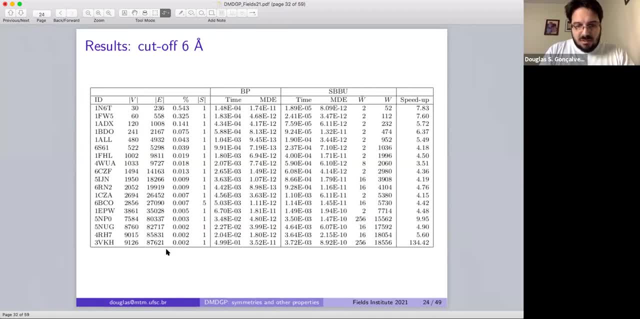 and prune And we compare it in two sets of proteins, okay, with cutoff distance of six angstroms. And so here you can see the number of atoms, the number of edges- I mean almost concluding Antonio- the number of sets, the number of eggs, the density of 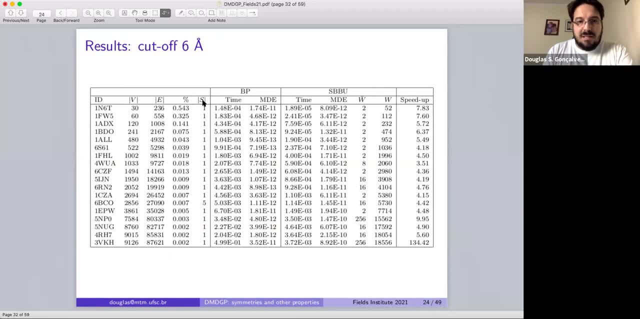 the graph, Okay, Here The cardinality, Okay, And here you can see the number of the sets: S and you have the plastic branch and prune and the new algorithm here have the time in seconds, So both are really really fast. 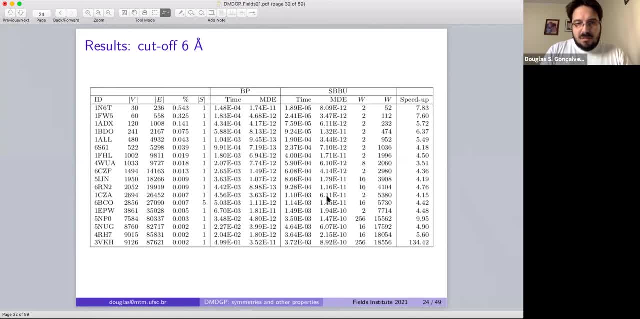 And the MDE is okay, very reasonable for order 10 to the minus 11, minus 12.. And we see that they speed up with the new algorithm with respect to BP is non-trivial. Okay, We we see that for some instances. 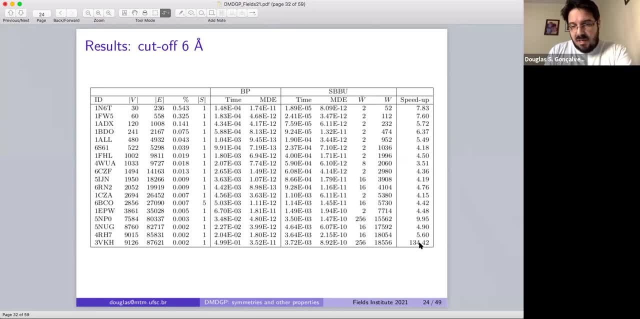 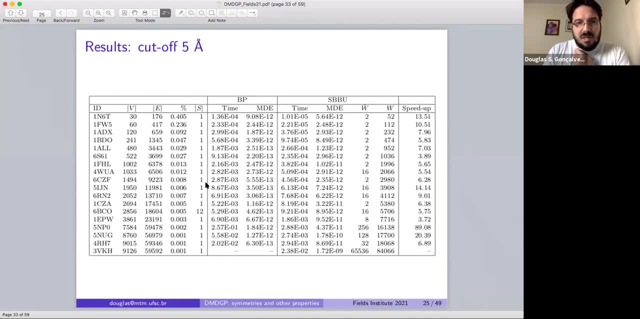 Okay, Okay, For some instances we have like hundreds of times faster than branch and prune, And the situation is also similar for sparser graphs. Okay, And in this case, in this particular case, we have one instance for which the branch 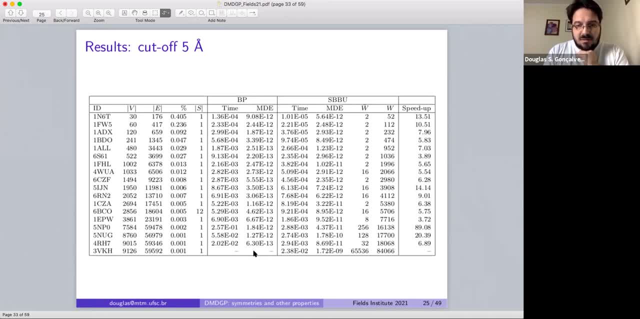 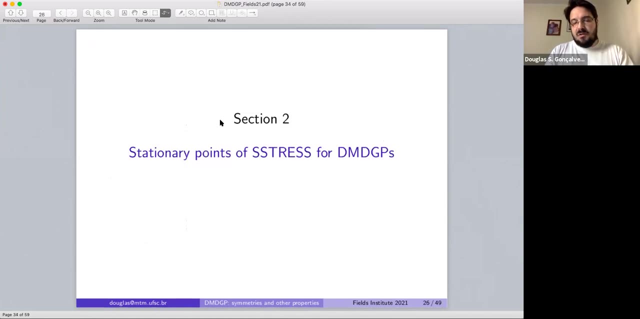 and prune could not find a solution in less than 300 seconds, which is this last one And for which we could find a solution. And here are. they speed up the ratio between the time of SBBU and SB. So In the second part of the book I would like to discuss the stationary points of the stress. 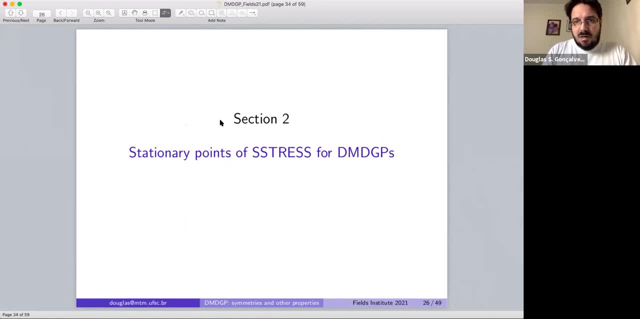 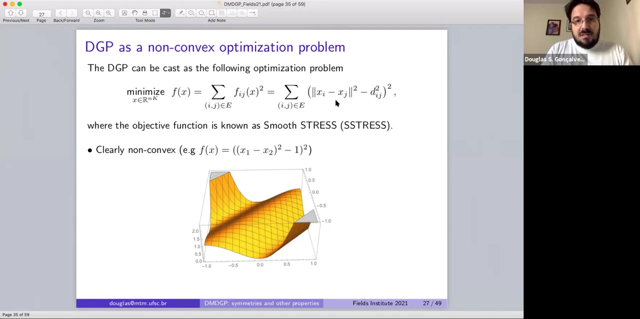 for DMG piece, but I think I run out of the time. Okay, I will only mention one last example, So let me just talk tell about the problem. So the problem is the following: that the decision problem can be formulated as a optimization. 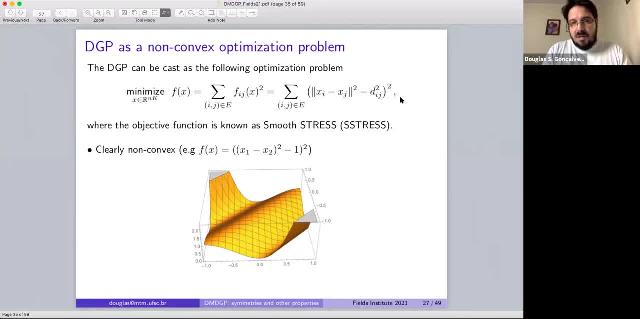 problem- I know linearly square problem given by this function In the literature. It's a problem In the literature of multinational scaling. this function is known as the smooth stress And there is an open question about the existence or not of local, non-global minimizers of this. 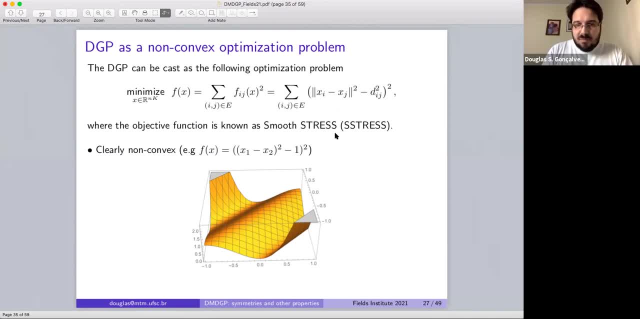 function Okay, But this is just a preliminary study from my side, So I will not go into details. I would just say that. So the question is that any non-global minimizer I'm not aware of, uh, um, any author who was? 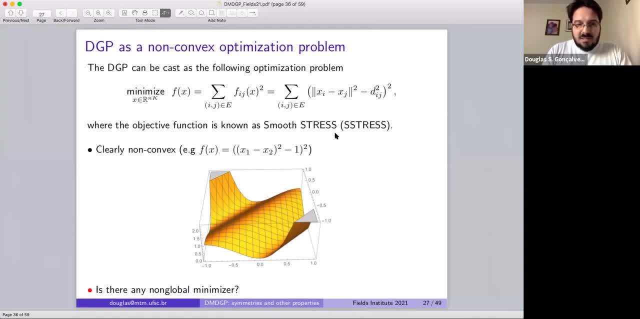 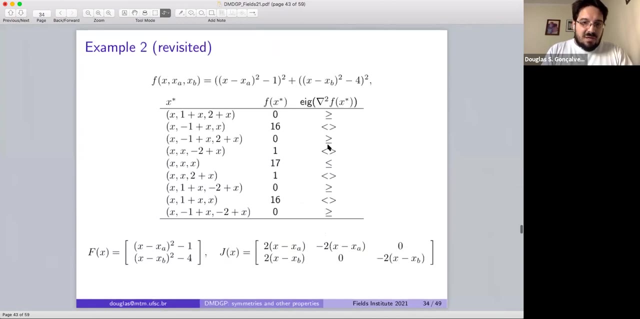 able to Uh analytically prove the existence of uh non-global minimizer for the smooth stress, not the stress. the smooth stress function Okay And I just like to say that, uh, okay For the DMGP. uh, we may have an example of uh local minimizer which is not global. 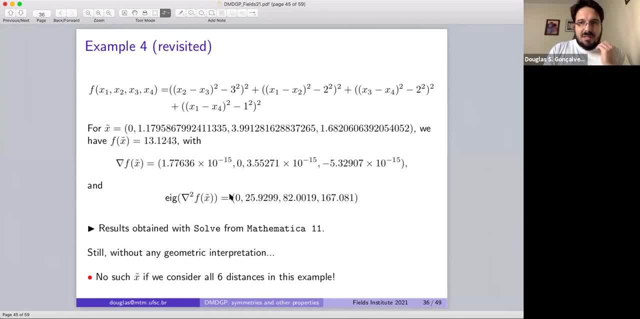 that I give here in the last slide. Uh, okay, These numbers are uh really large here because actually our, our numerous size. Okay, This is the result of my computations, My algebraic computations, with this, the, the Mathematica. 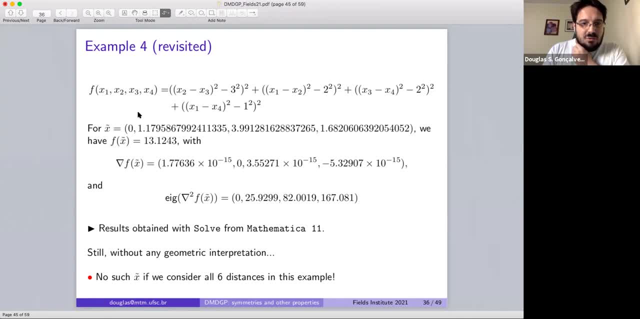 Okay And uh, we managed to show that the for this instance of the DMGP in dimension one, we do have a local minimizer, or at least it seems so. but there is a trick here, because we do not have all the distances available. 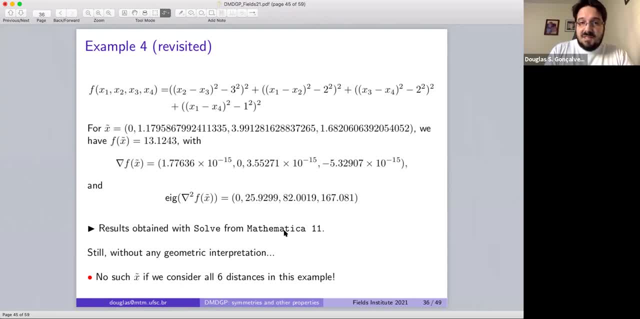 Okay, We have four points, but only for distance instead of six. If you include the other six, Okay, Six distance- then the, the local minimizer disappears, And so we still have this open question with, I hope someone here in the audience, uh, can. 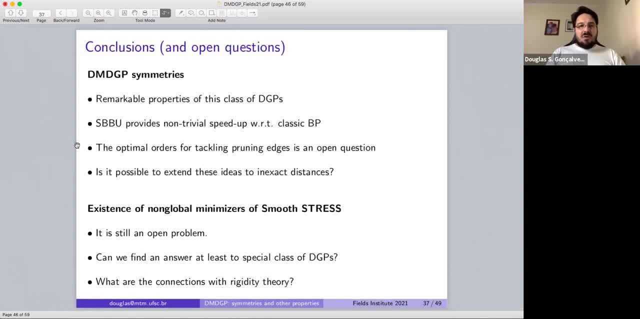 help me with uh. I don't know some reference And so in conclusion I'd like to say that the discretized one, molecular decision problems. they have very interesting and remarkable symmetry properties, uh, which may be exploited to solve problem more efficiently, in particular. 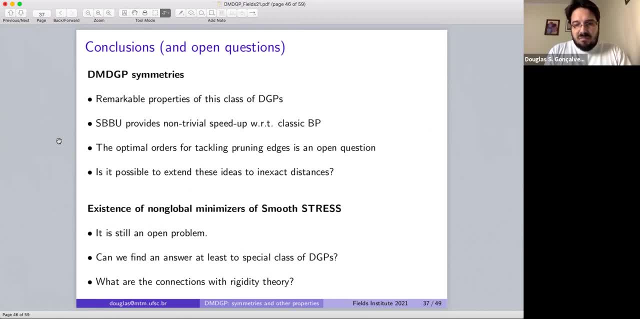 Okay, So this allows us to count the number of solutions of the problem without needing to solve the problem. Uh, they also, uh, tell us that, given one solution, I can generate all the orders. Okay, By using partial reflections and exploiting the symmetry properties, we were able to. 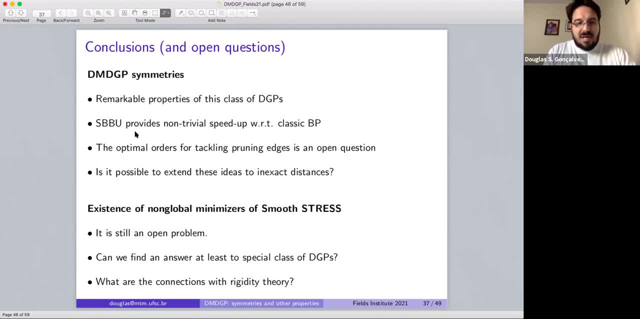 um, to present a new algorithm for this class of decision problems which has um, um- how can I say? Uh, a considerable or A non-trivial speed up with respect to the classic branching prune. There are some open questions: the the specific order in which the pruning edge should be. 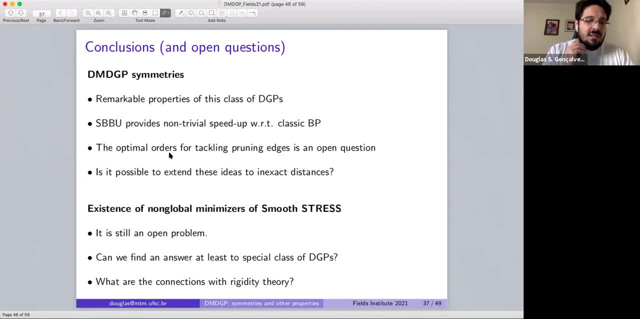 treated here. We treated them in- uh, let me remember- in increasing order of I and decreasing order of J. So we, if you imagine a distance matrix, we treat first the distance that are closer to the diagonal And then later the ones that are farther from the diagram. 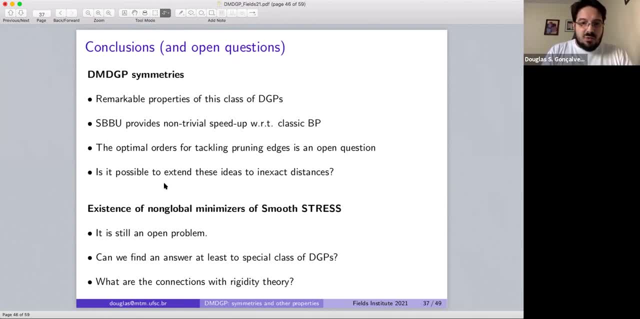 And, of course, a question: is it possible to extend these ideas to treat in exact distance- And we are still working on on this topic- and the concerning the existence of non-global minimizers of uh? is move stress function? Uh, I would say that is still an open problem. 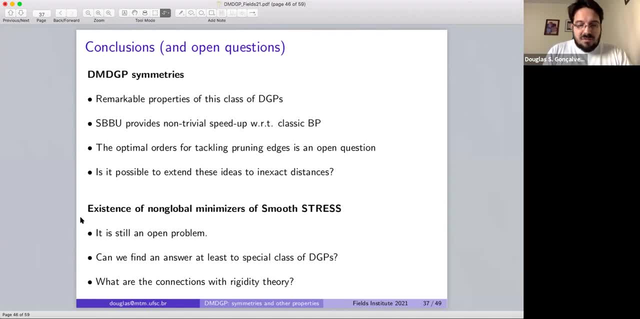 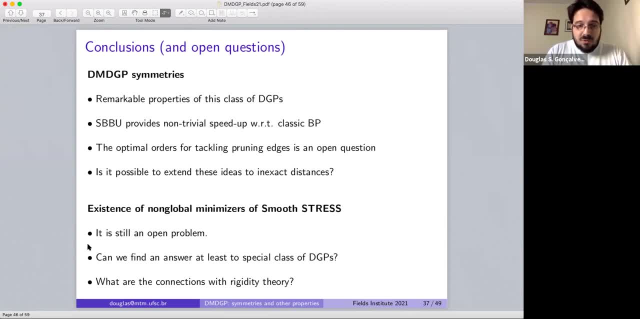 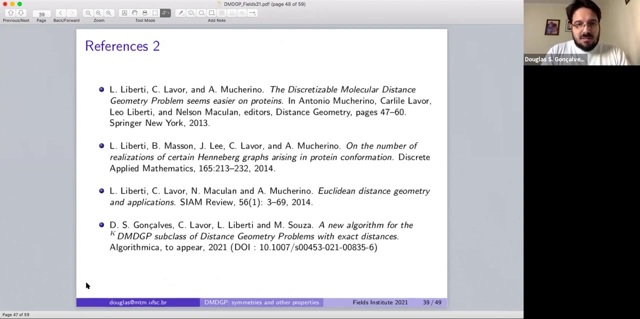 a local minimizer which is not global, as we could do in the last example of DMGP, but in that case we do not have all the distances. And what are the connections of this question with rigid theory? So here are some references that you can see later in the video and thank you for your 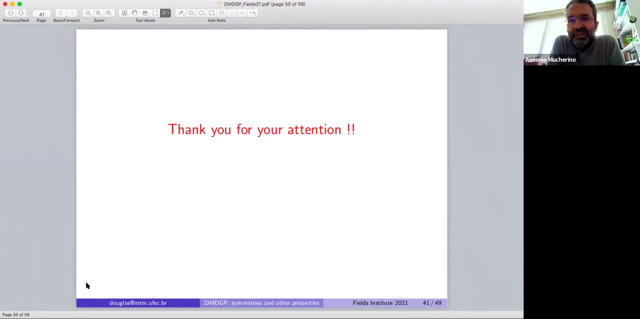 attention. Thank you very much, Douglas. So are there any questions? Maybe we have some some in the chat. let me just: yeah, there was. yeah, there was one left in the chat, Otherwise we have. So. 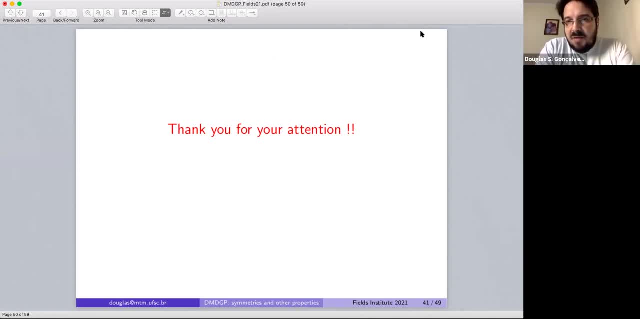 Itamar asked: are the reflections and partial reflections inducing symmetries? Yes, Itamar, it's exactly that. Yeah, the symmetries are induced by this partial, by the hyperplanes actually, but which are related to the partial reflection. 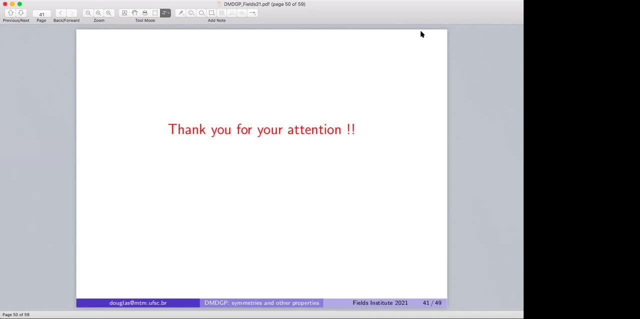 Another point is: how about reflect projections? If I choose the right or suitable plane hyperplane to reflect on, I may induce also some hidden symmetries or realistic protein symmetries, And So the question now is: you focused on reflections and partial reflections. 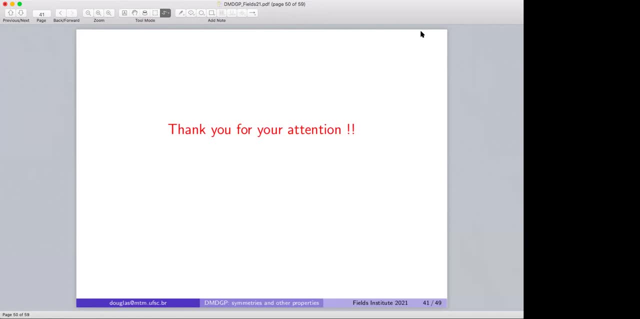 Yes, But the projections are also part of the toolkit. no, Yes, of course. of course, Indeed, you can. you can describe a reflection using projections. Okay, but For the DMA-DGP we only consider the partial reflections. 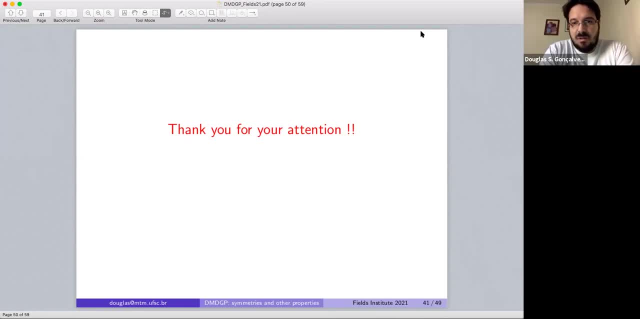 It was the- I don't know- the most natural operation to consider given the structure of our problem, But we may consider this idea. Okay, Other questions From the audience? Yes, What about the noise data, Henry? Yeah, 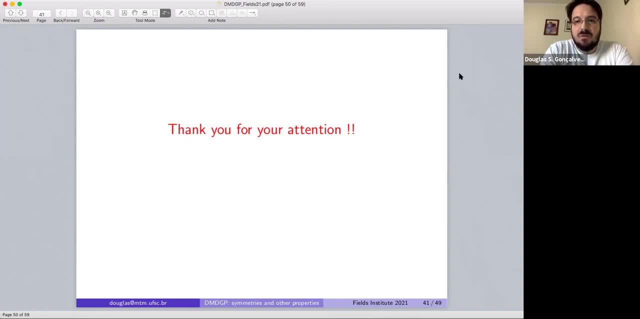 So we we still do not have conclusive results using noisy data. So, to begin with, we we cannot show the same properties I presented today If we consider the data are noisy. And perhaps the first question when we are dealing with this: 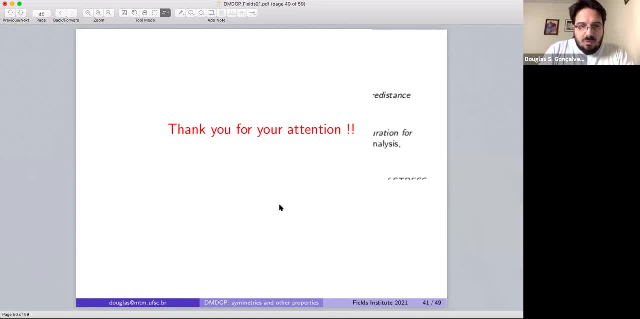 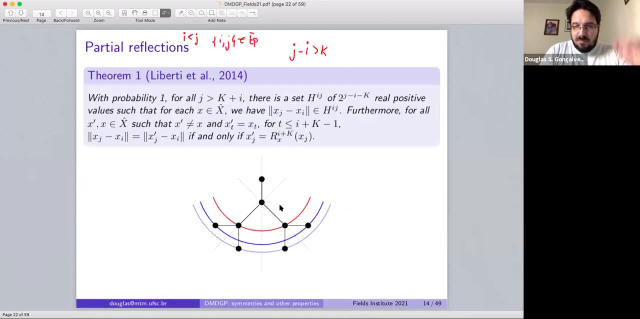 symmetries is which candidate configuration should we choose? So let me show the my repeated picture here. So let's suppose that this, I don't know- the light blue distance is correct, But now it is corrupted by noise. Okay, So in this case, none of the. if you, if you consider epsilon, zero tolerance. 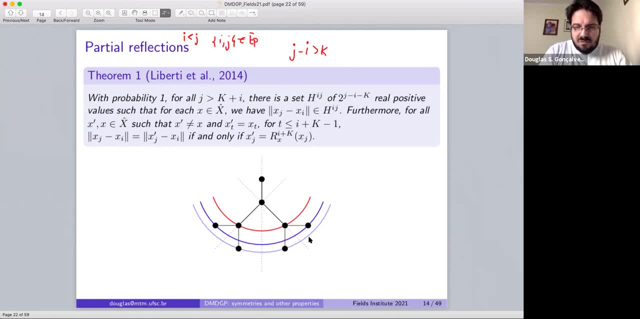 none of the candidate realizations for the vertex four will fulfill this. this distance Okay. And then, if we consider this a search in the tree, we would stop. But then one could say, okay, so consider the right. 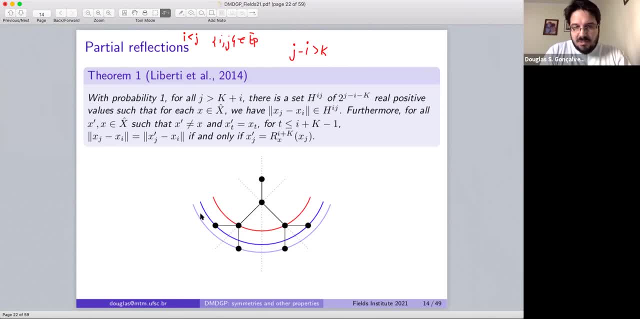 candidate realization, the one which minimizes the violation of this noise distance. Okay, But then in this case we can maybe come up with a noisy distance for which all the four positions here will be accepted, And so we needed to. 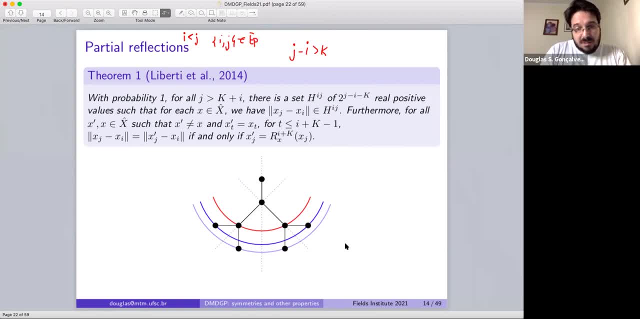 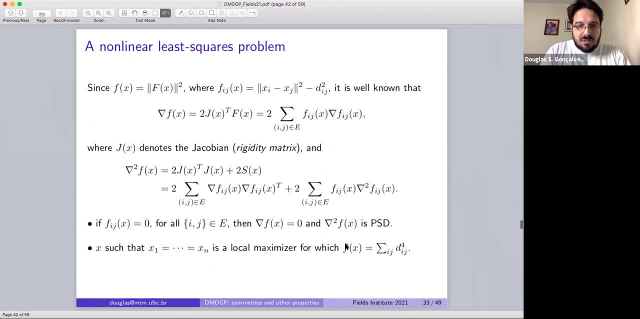 to change the theorems and the structure of the algorithms and so on. What I can say, Henry, from our group, okay, including Leo, Carlile, Antonio, Michael, we've done some advances in this direction. Where is it? 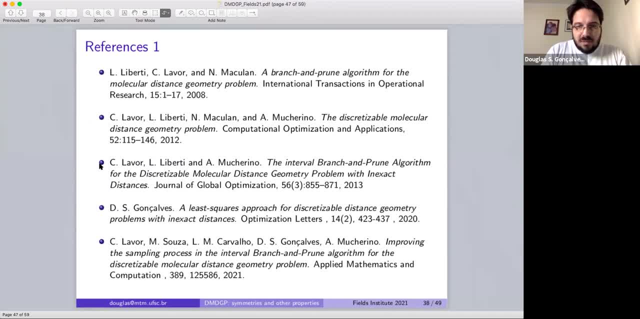 Considering interval distances. So in this paper, okay, of Carlile Leo and Antonio and this paper by myself, in this one they considered the inexactness modeled by an interval and then sample this interval. But then 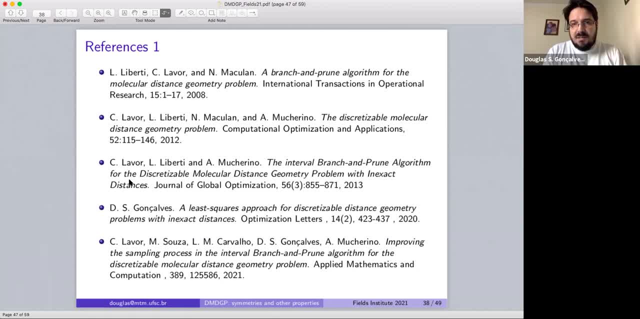 the. the search tree is no longer binary, but or. K is the number of samples you choose. Okay, And the results are not that good. We could only have good results for small proteins In this paper. I consider a sort of least square approach for the problem. 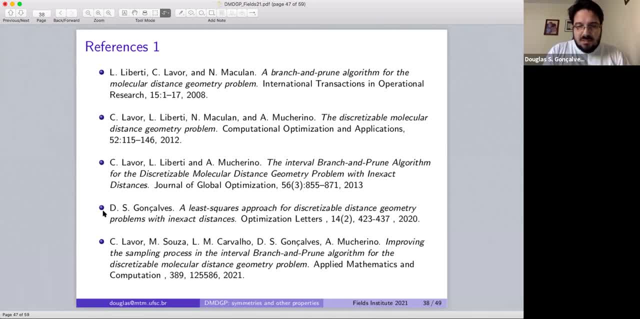 So here I consider the distance as it is with noise, And then the difference with respect to the branch and prune is that here I use the Euclidean distance matrix approach to solve the subproblems in a least square sense. Okay, 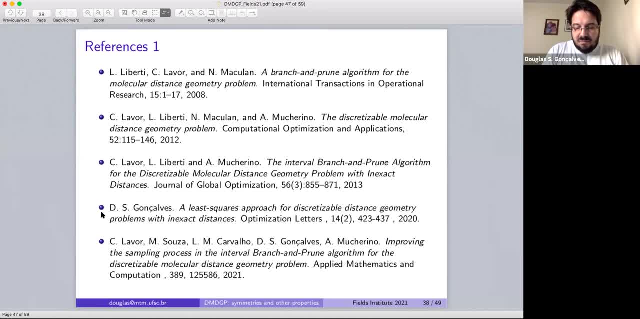 And I keep track of the eigenvalues, of the partial realizations, And they say, oops, we are in our tree. If the fourth eigenvalue is much, much larger than a certain threshold, something is wrong. I prune it backtrack. 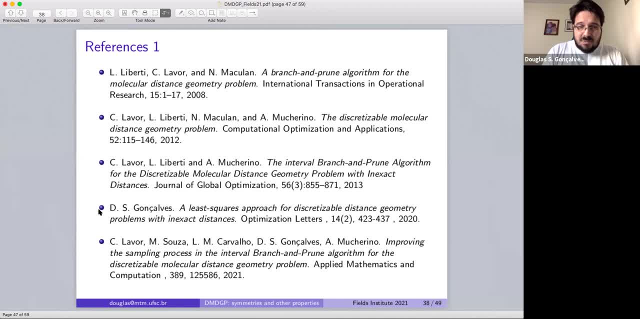 And here we could get kind of nice results, but only for very small noise, Henry. I would say at most one or 2% multiplicative noise. All right, Yeah, I guess the noise starts growing after, Exactly. 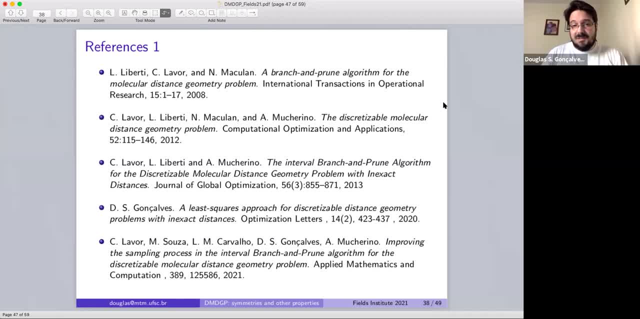 Yeah, And it's a sequential method And it's, I think, that noise it's even worse for sequential methods, for buildup methods.